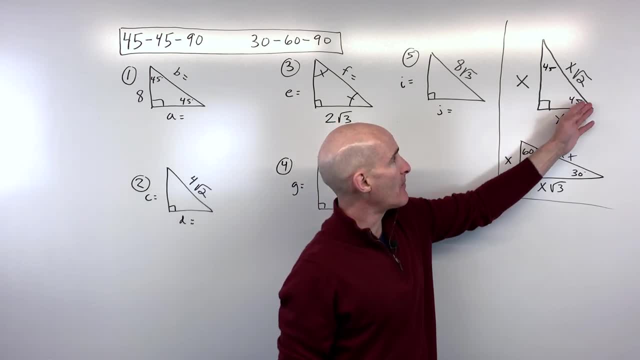 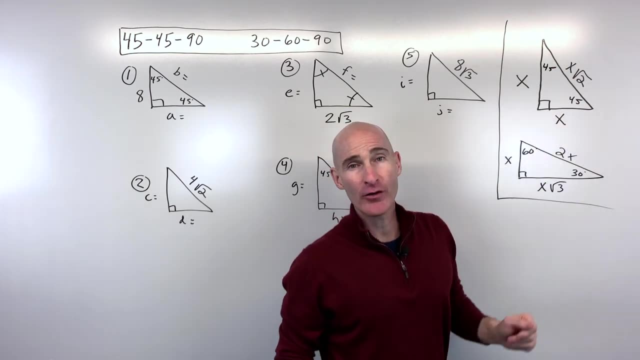 note square root of 2, it's about 1.2.. Which means that the hypotenuse is about 1.4 times longer than the leg. It's just that when we multiply by square root of 2, we're getting an exact value for that hypotenuse. So let's. 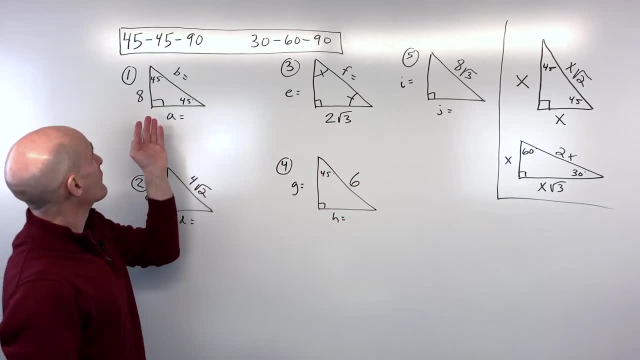 jump into some examples, see if you can try some of these on your own as well. But for the first one, you can see they're giving us this 45-45-90 triangle and they're giving us a leg or a side. 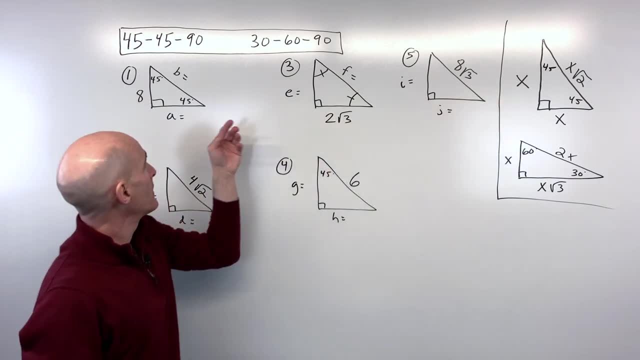 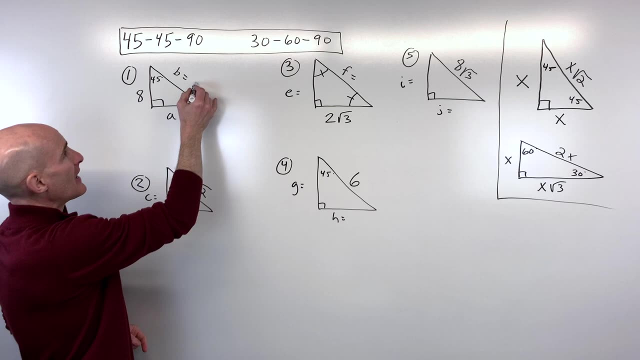 of 8.. So you can see, x is equal to 8, which means that a over here, this other leg, must also be 8.. And if we want to find the hypotenuse, we just take the leg and we multiply by the square root. 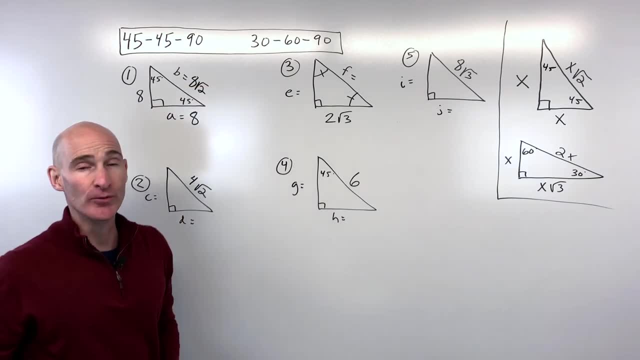 of 2.. So side b, here the hypotenuse is going to be 8 root 2.. Now let's go to another example, Number two. here we've got a 45-45-90.. And sometimes they'll denote that by showing you. 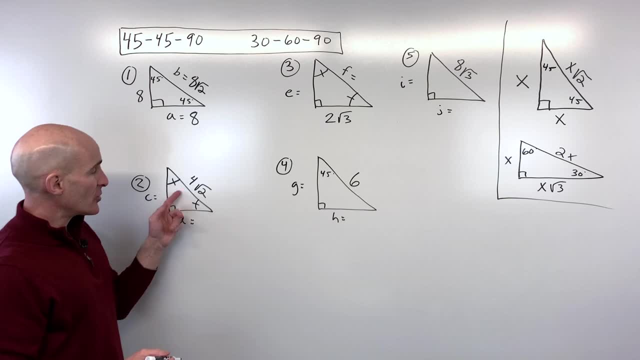 that these two acute angles are congruent. And that's how you know. it's a 45-45-90.. But you can see they're giving us the hypotenuse. So here what we want to do to get back to the leg. 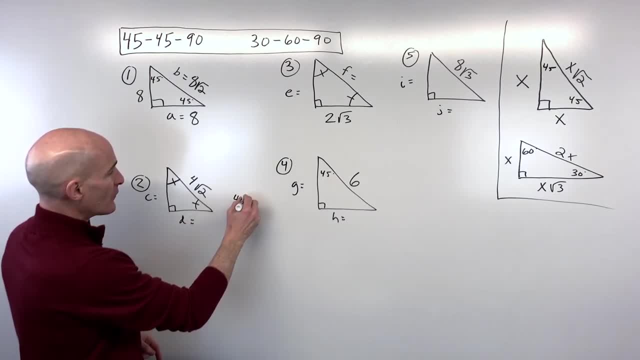 is we're going to want to divide by the square root of 2.. So if we take 4 root 2, divided by square root of 2, those square root of 2's cancel out and we're just left with 4.. 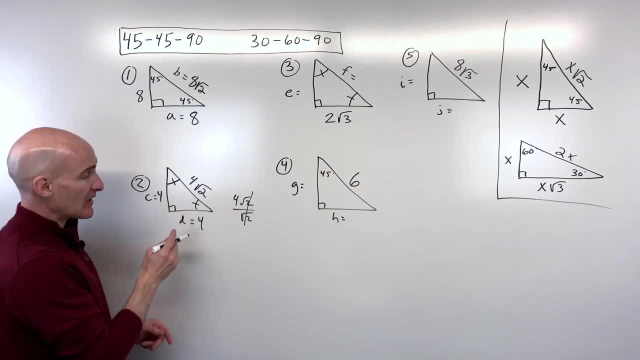 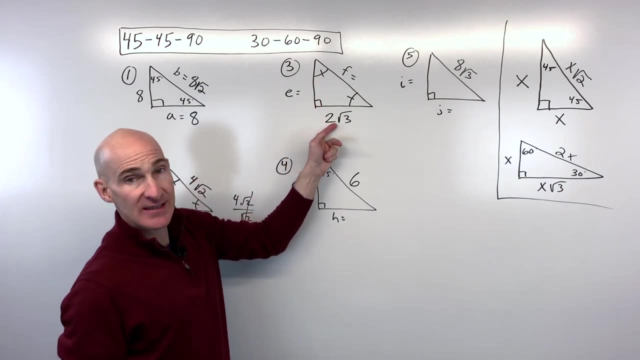 And remember, in a 45-45-90,, these two legs that make up that right angle are going to be congruent. Okay for number three. now, same thing, 45-45-90,. they're giving us the leg as 2 root 3, which means 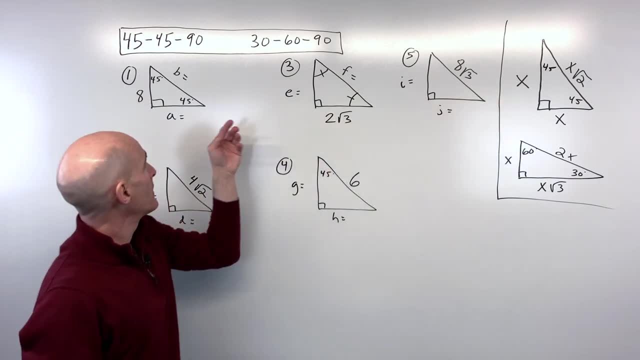 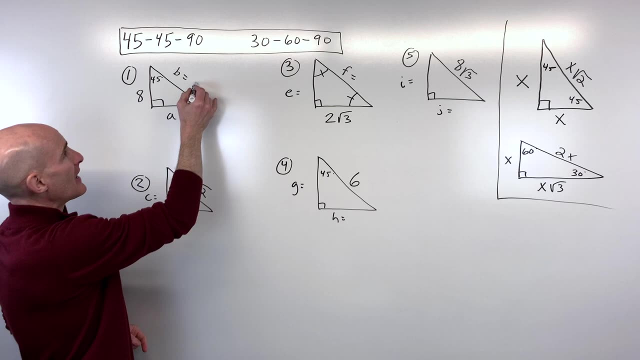 of 8.. So you can see, x is equal to 8, which means that a over here, this other leg, must also be 8.. And if we want to find the hypotenuse, we just take the leg and we multiply by the square root. 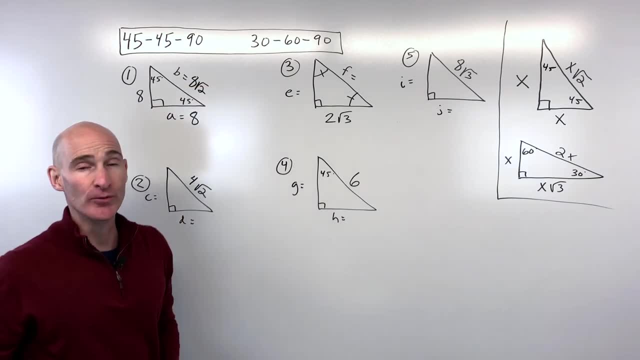 of 2.. So side b, here the hypotenuse is going to be 8 root 2.. Now let's go to another example, Number two. here we've got a 45-45-90.. And sometimes they'll denote that by showing you. 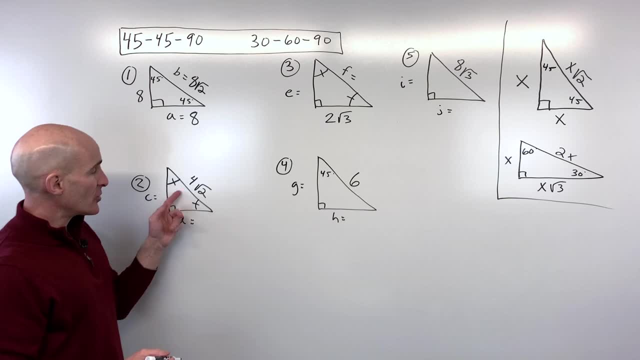 that these two acute angles are congruent. And that's how you know. it's a 45-45-90.. But you can see they're giving us the hypotenuse. So here what we want to do to get back to the leg. 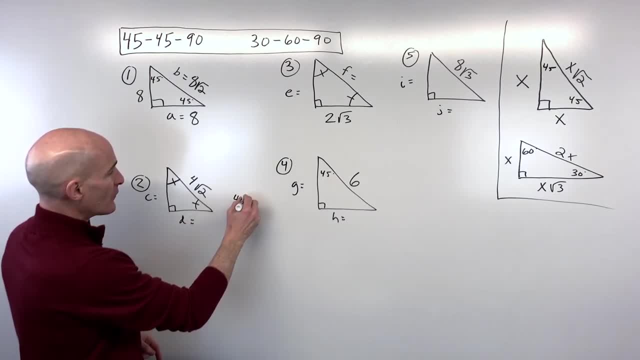 is we're going to want to divide by the square root of 2.. So if we take 4 root 2, divided by square root of 2, those square root of 2's cancel out and we're just left with 4.. 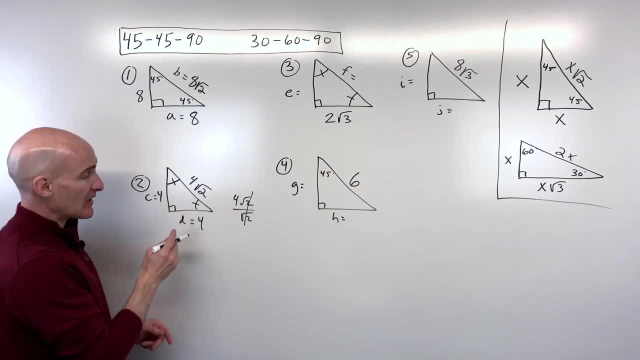 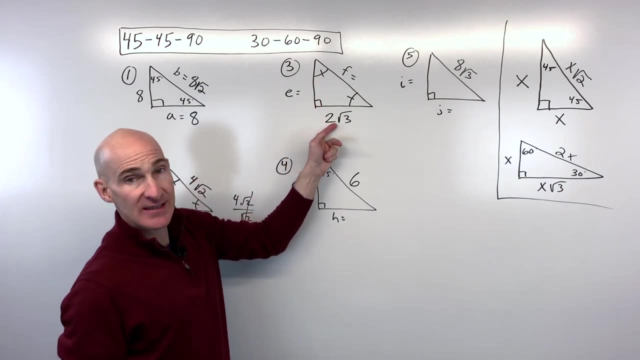 And remember, in a 45-45-90,, these two legs that make up that right angle are going to be congruent. Okay for number three. now, same thing, 45-45-90,. they're giving us the leg as 2 root 3, which means 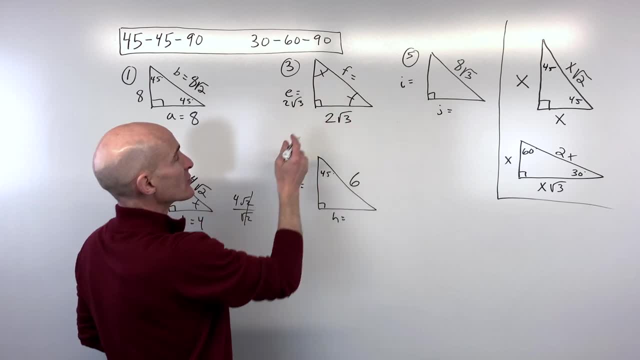 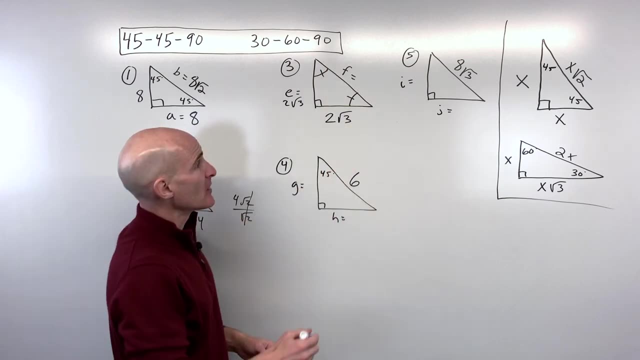 that this other leg over here must be 2 root 3, since the legs are congruent. But to get to that hypotenuse we have to multiply by the square root of 2.. Remember, it's about 1.4 times longer. So if we 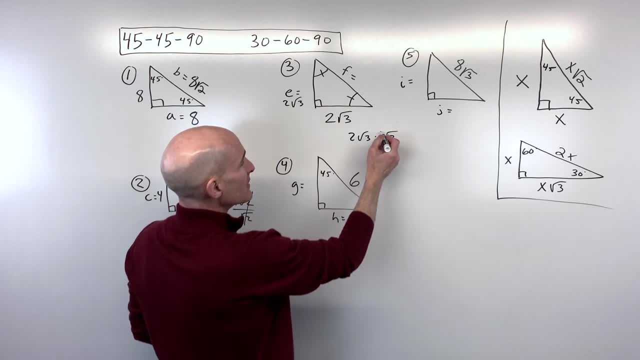 multiply by 2 square root of 3 times square root of 2, you can think of this as like 1 square root of 2.. You multiply the integers together and the square roots together. So 2 times 1 is 2, square root of 3. 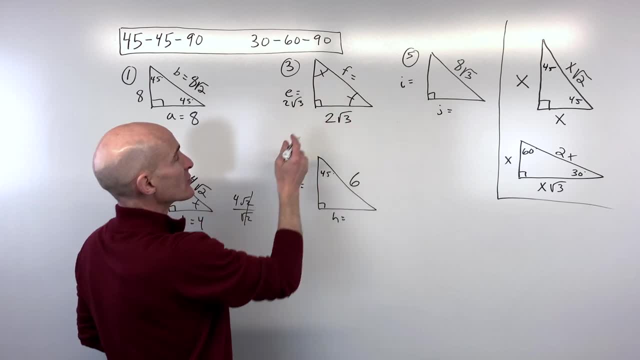 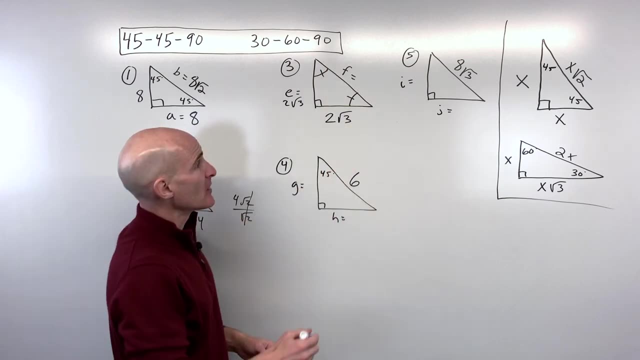 that this other leg over here must be 2 root 3, since the legs are congruent. But to get to that hypotenuse we have to multiply by the square root of 2.. Remember, it's about 1.4 times longer. So if we 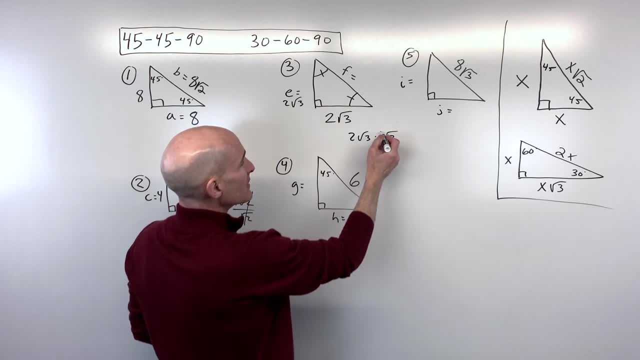 multiply 2, square root of 3 times square root of 2, you can think of this as like 1 square root of 2, you multiply the integers together and the square roots together. So 2 times 1 is 2.. Square root of 3. 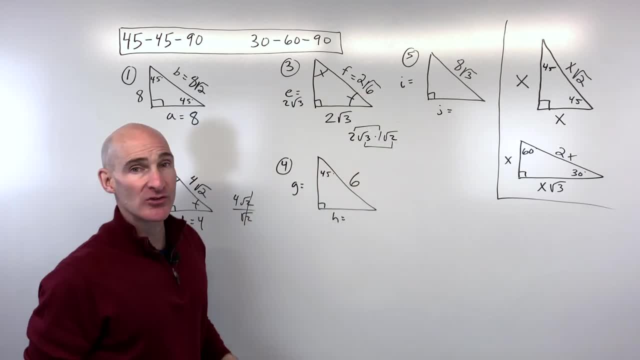 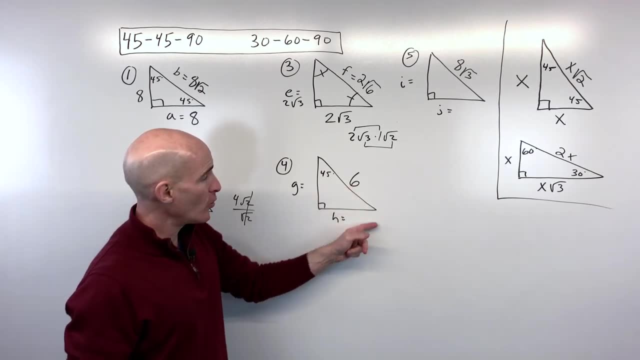 times, square root of 2 is square root of 6. And that's going to be your hypotenuse. Okay, for number 4,, again we have a 45-45-90.. They're giving us the hypotenuse now is 6.. We have to make our way back. 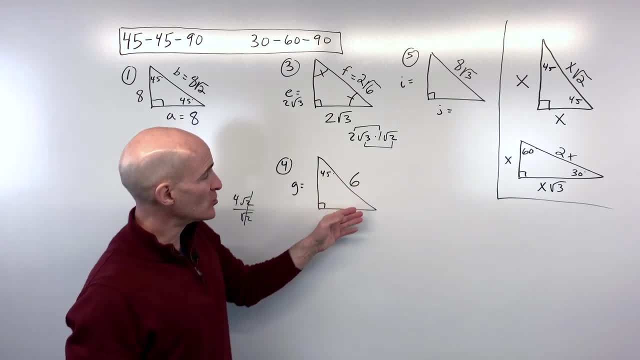 to the leg. So remember, the hypotenuse is square root of 2 times longer than the leg. So to go back to the leg, we have to multiply by the square root of 2.. And we don't want that square root of 2 in the denominator, That's: 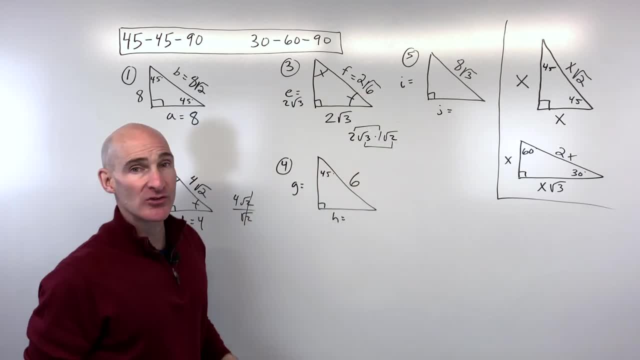 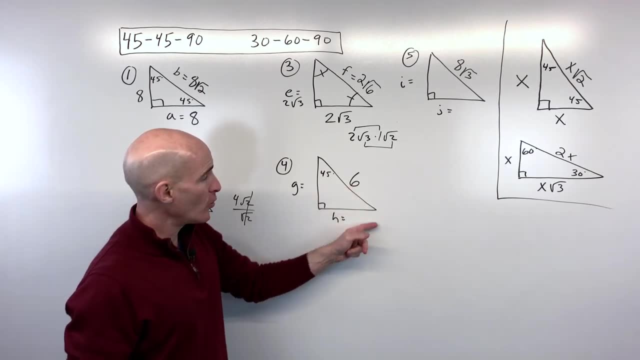 times, square root of 2 is square root of 6. And that's going to be your hypotenuse. Okay, for number 4,, again we have a 45-45-90.. They're giving us the hypotenuse now is 6.. We have to make our way back. 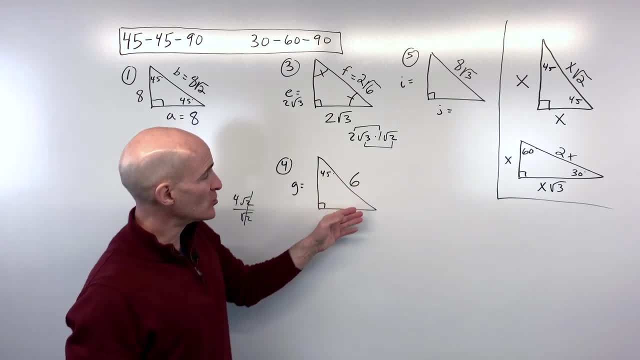 to the leg. So remember, the hypotenuse is square root of 2 times longer than the leg. So to go back to the leg, we have to multiply by the square root of 2.. And we don't want that square root of 2 in the denominator, That's: 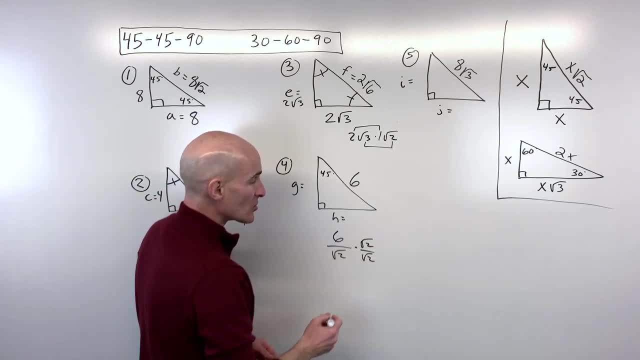 considered improper. So what we're going to do is we're going to do a process called rationalizing, where we multiply the numerator and denominator by square root of 2.. That's like multiplying by 1.. And so if we multiply horizontally across, we get 6 square root of 2.. Square root of 2 times square root of 2. 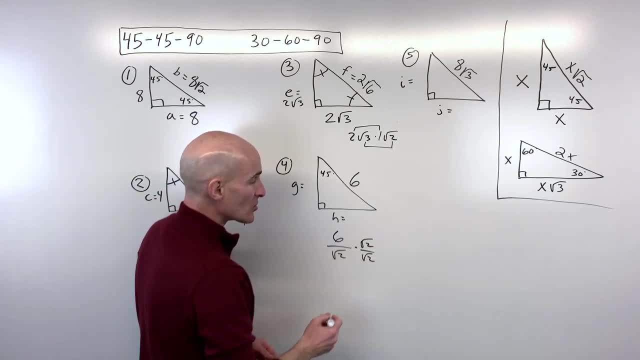 considered improper. So what we're going to do is we're going to do a process called rationalizing, where we multiply the numerator and denominator by square root of 2.. That's like multiplying by 1.. And so if we multiply horizontally across, we get 6 square root of 2.. Square root of 2 times square root of 2. 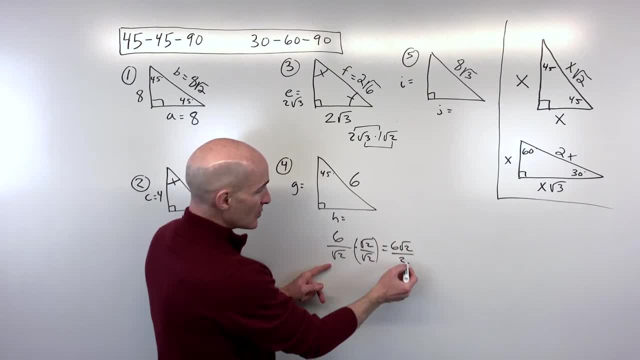 is square root of 4, which is just equal to 2.. And then you can see the 6 and the 2 reduce and that's giving us 3 square root of 2.. So that's going to be this leg as well as this leg, because 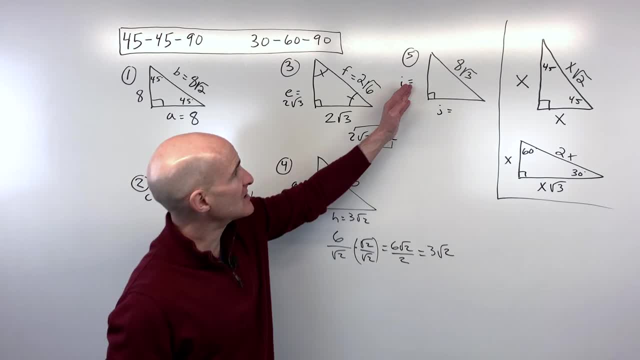 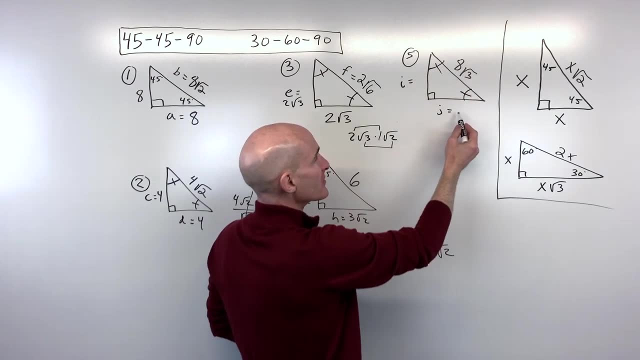 the legs are congruent. Okay, last 45-45-90 example, a little bit more challenging. Here you can see that we've got. the hypotenuse is 8 root 3. We want to go back to the leg, So 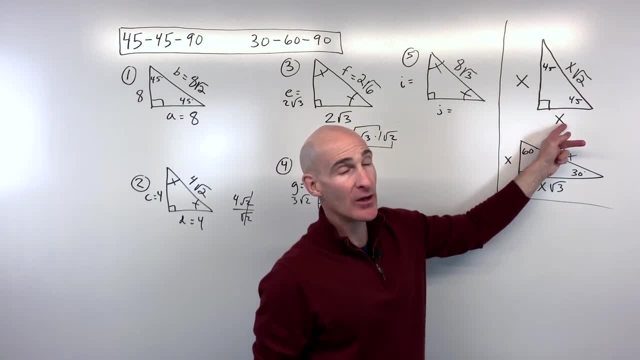 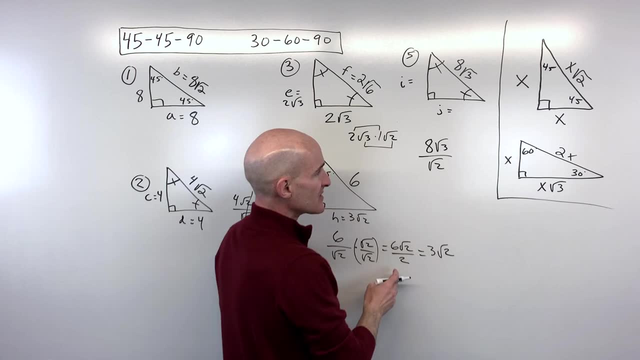 remember, when you're going from the x root 2 side, the hypotenuse to the leg, we have to divide by the square root of 2.. So here we've got 8 square root of 3 divided by square root of 2.. Just like this. 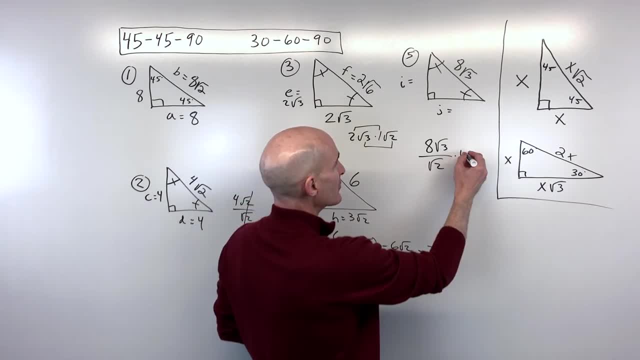 last problem: we didn't want the radical in the denominator, the square root of 2 in the denominator. So we're going to multiply the top and bottom by square root of 2.. Remember you multiply the numbers together and the square roots together, So that's going to be 8 square root of 6. 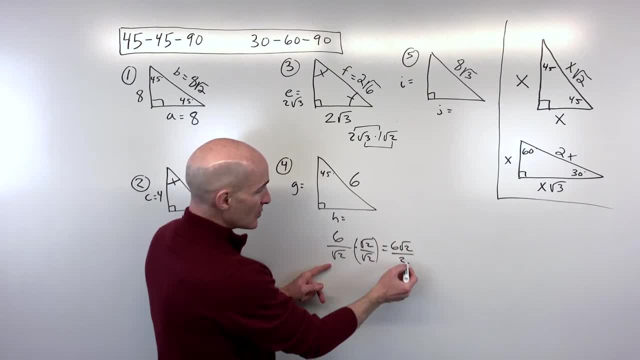 is square root of 4, which is just equal to 2.. And then you can see the 6 and the 2 reduce and that's giving us 3 square root of 2.. So that's going to be this leg as well as this leg, because 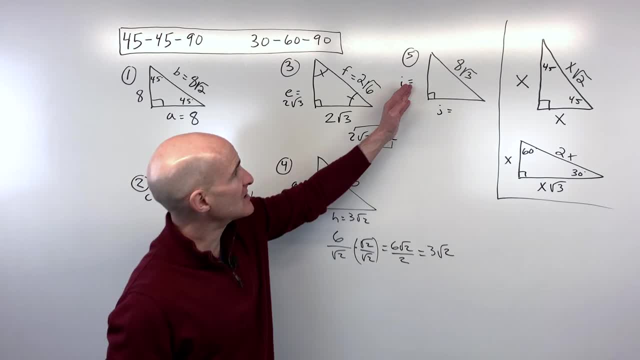 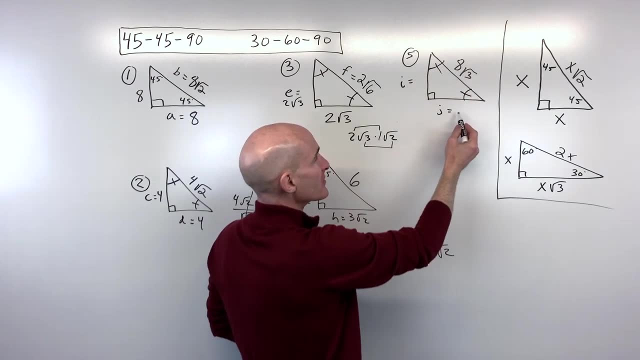 the legs are congruent. Okay, last 45-45-90 example, a little bit more challenging. Here you can see that we've got. the hypotenuse is 8 root 3. We want to go back to the leg, So 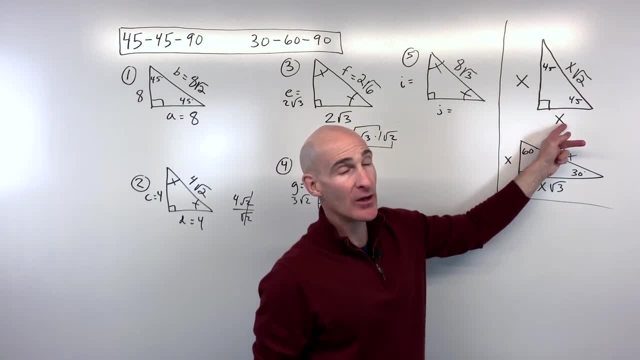 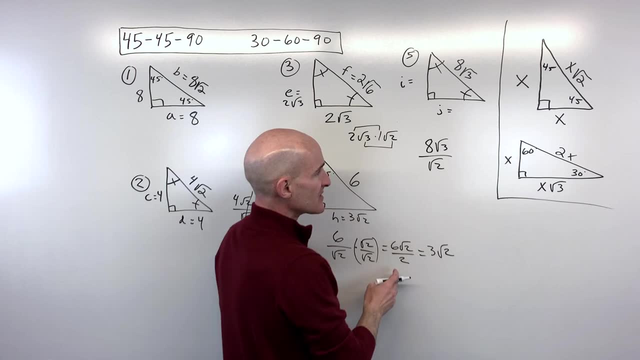 remember, when you're going from the x root 2 side, the hypotenuse to the leg, we have to divide by the square root of 2.. So here we've got 8 square root of 3 divided by square root of 2.. Just like this. 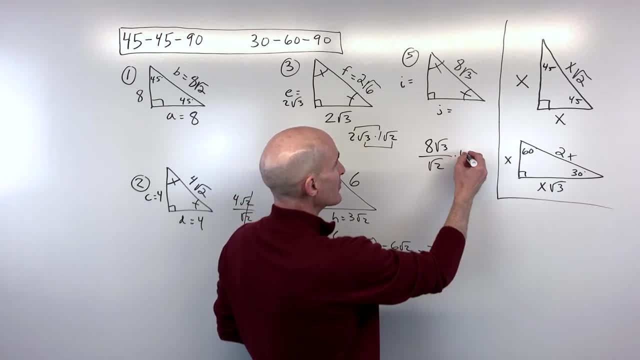 last problem: we didn't want the radical in the denominator, the square root of 2 in the denominator. So we're going to multiply the top and bottom by square root of 2.. Remember you multiply the numbers together and the square roots together, So that's going to be 8 square root of 6 all over. 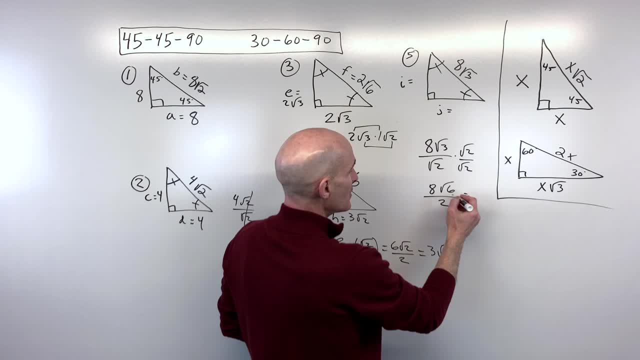 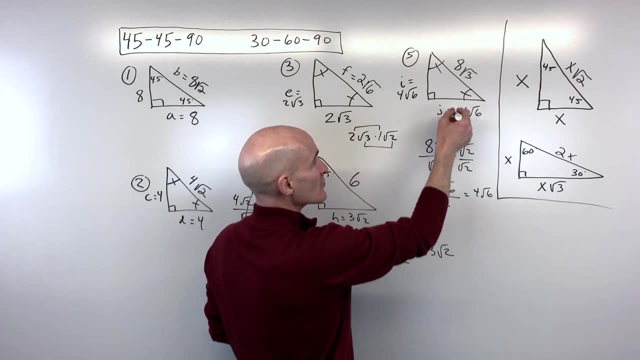 square root of 4, which is 2.. The 8 and the 2 we can reduce, 2 goes into 8 four times. So we get 4 square root of 6 for j and 4 square root of 6 for i, because remember, the legs are congruent. Okay. 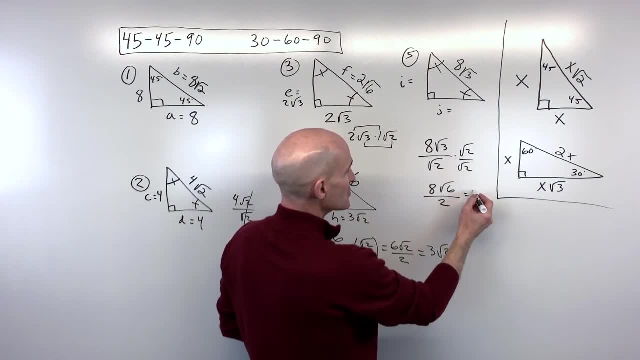 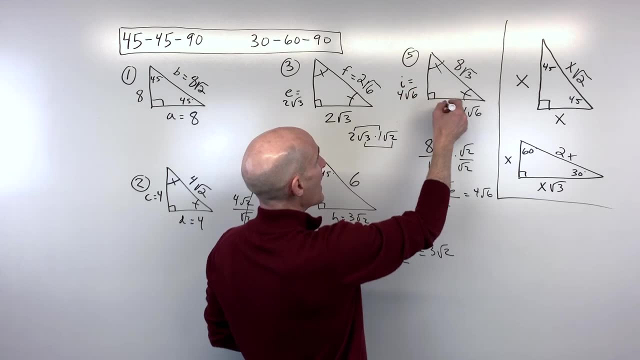 all over square root of 4, which is 2, the 8 and the 2 we can reduce, 2 goes into 8 four times. so we get 4 square root of 6 for J and 4 square root of 6 for I, because, remember, the legs are congruent. 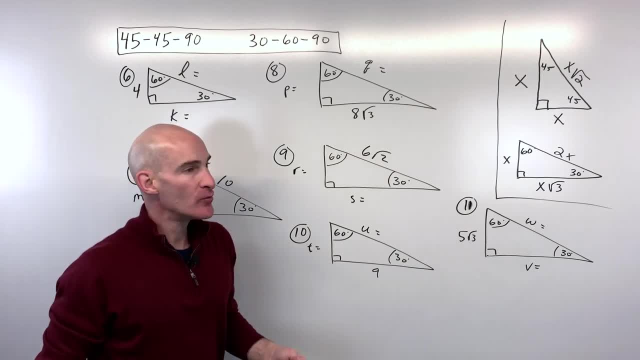 Okay, now the 30-60-90 Triangle. A little more challenging, but not too bad. What you want to remember here with the 30-60-90 is that across from the 30 degree angle, that's going to be the 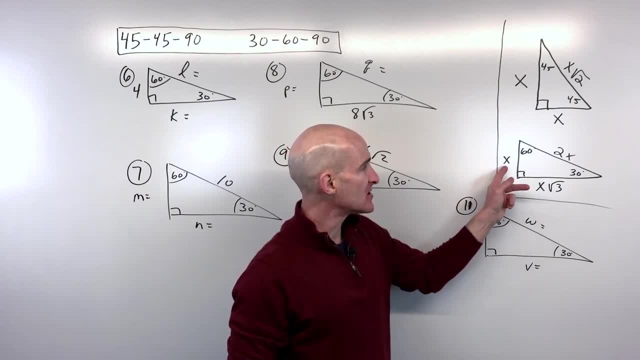 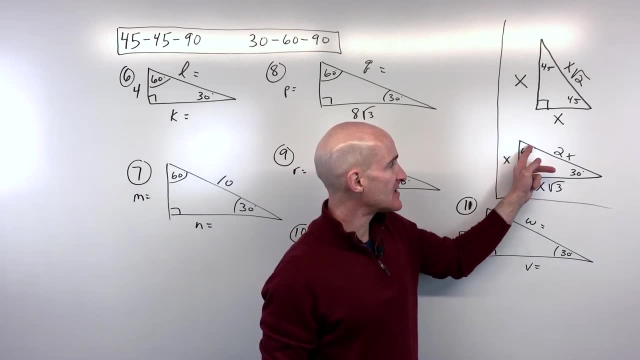 shortest side. That's the shortest leg And we call this the light side. that leg x. the one across from the 60 degree angle, that's the longer leg, that's x times the square root of 3, and the one across from the 90, that's the hypotenuse. that's the longest side. 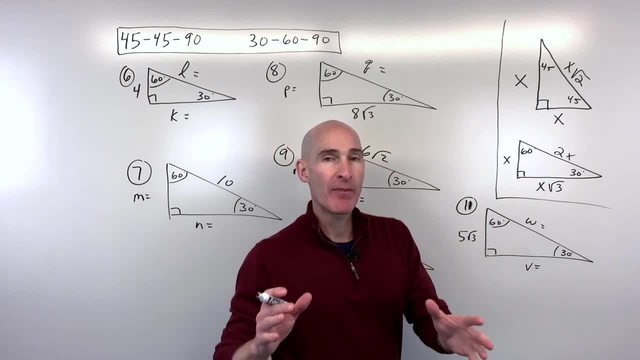 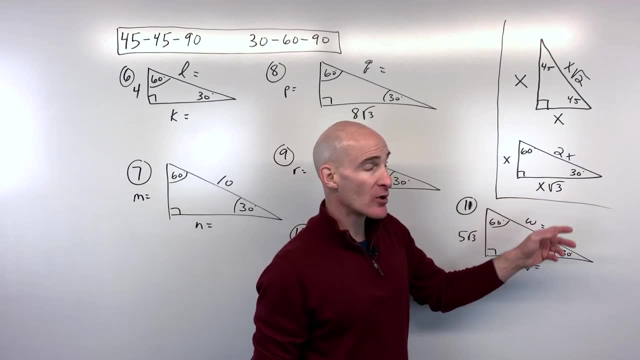 that's 2x. Now just a quick note: square root of 3 is about 1.7, so if you're going from the shorter leg to the longer leg, you're basically multiplying by 1.7. the only thing is that square root 3 is. 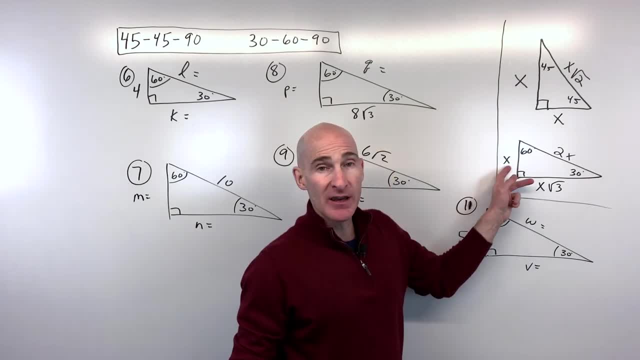 going to give you an exact value for that leg. So the way I like to think about it- and you can think about this as well- is: if you have the shorter leg, it's an easy problem. you just have to double it to get the hypotenuse, or multiply by square root of 3 to get the longer leg. If they 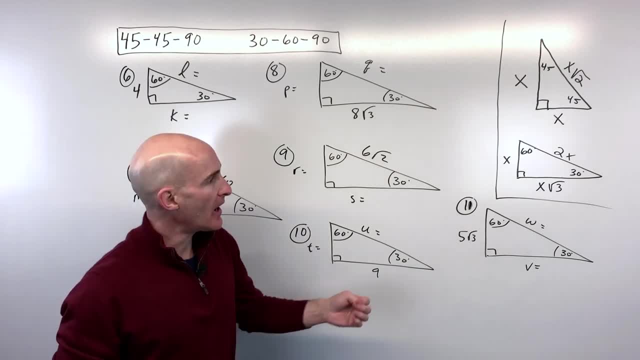 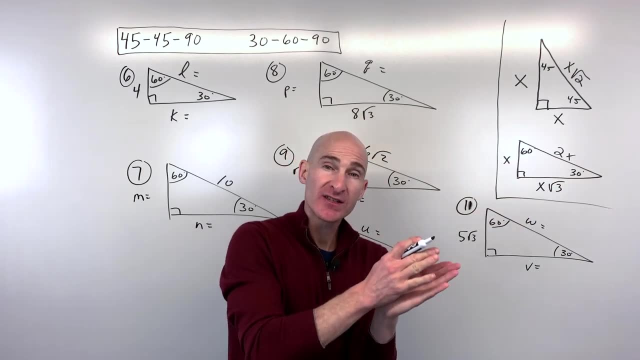 now the 30-60-90 triangle. A little bit more challenging, but not too bad. What you want to remember here with the 30-60-90 is that across from the 30 degree angle, that's going to be the shortest side, That's the shortest leg, And we call that the 30-60-90 triangle. So we're going to go. 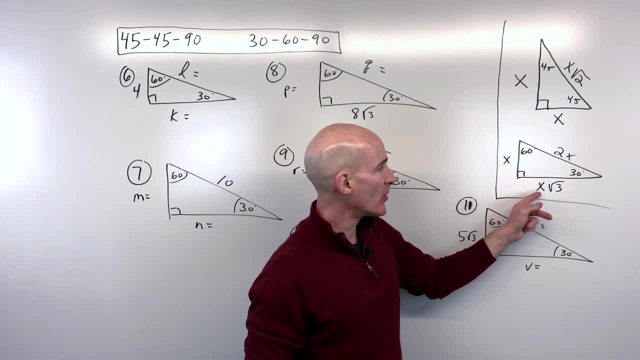 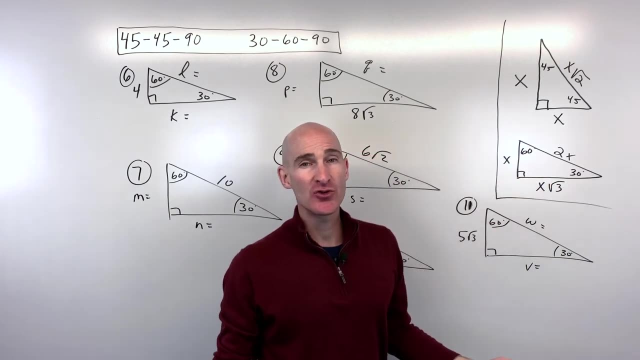 across from the 60 degree angle. that's the longer leg, that's x times the square root of 3.. And the one across from the 90,, that's the hypotenuse, that's the longest side, that's 2x. 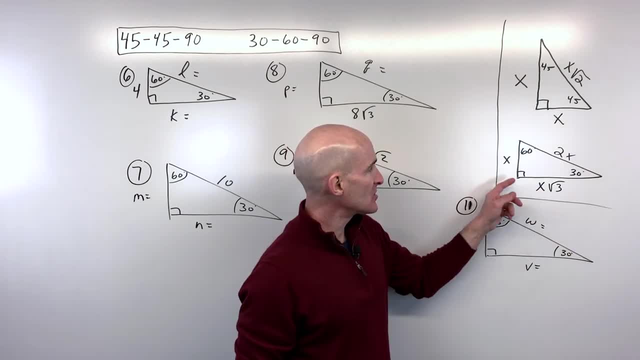 Now just a quick note. square root of 3 is about 1.7.. So if you're going from the shorter leg to the longer leg, you're basically multiplying by 1.7.. The only thing is that square root 3 is going. 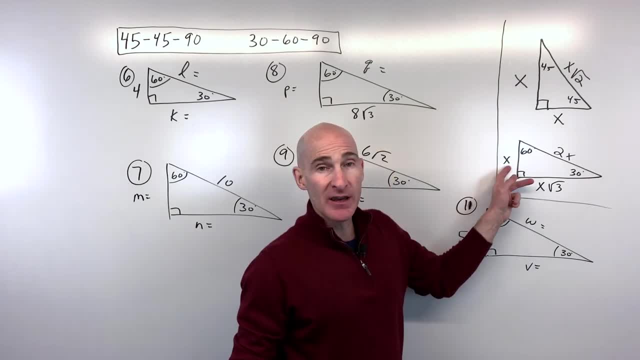 to give you an exact value for that leg. So the way I like to think about it- and you can think about this as well- is: if you have the shorter leg, it's an easy problem. You just have to double it to get the hypotenuse, or multiply by square root of 3 to get the longer leg. If they give you. 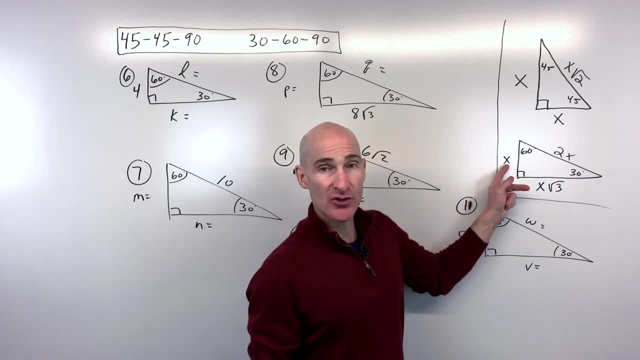 the hypotenuse. it's still a pretty easy problem. You just divide by 2 to get the shorter leg and then multiply by square root of 3 to get the longer leg. The tougher one sometimes is if they give you this longer leg, you're going to have to divide by square root of 3 to get back to that shorter leg. 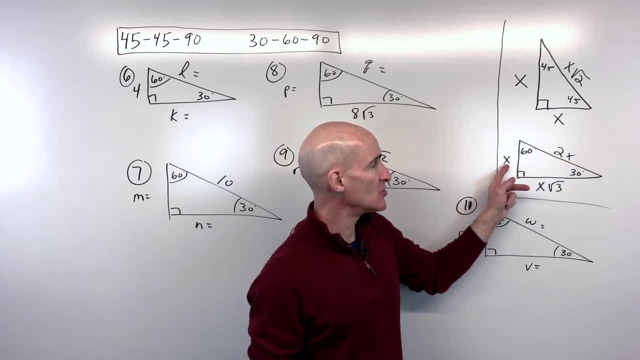 give you the hypotenuse, it's still a pretty easy problem. you just divide by 2 to get the shorter leg and then multiply by square root of 3 to get the longer leg. The tougher one sometimes is, if they give you this longer leg, you're going to have to divide by square root of 3 to get back to that. 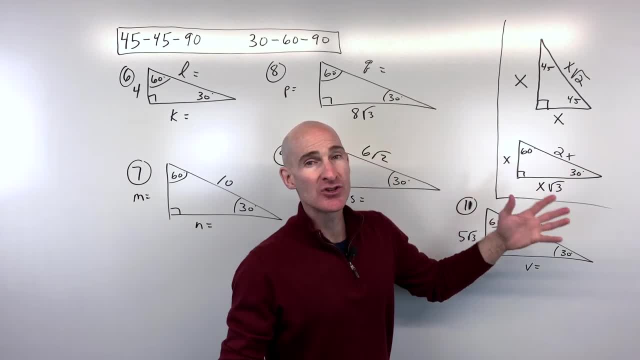 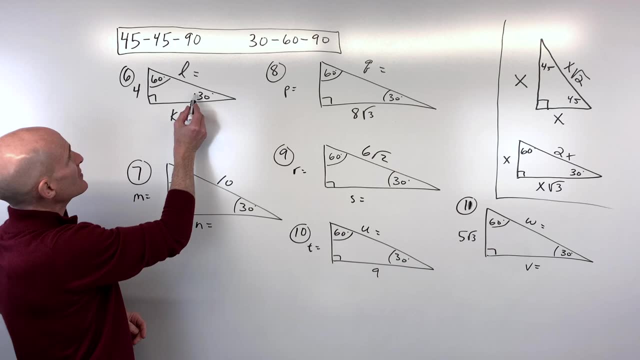 shorter leg and then double it to get the hypotenuse. So let's go through some examples so you can see how this works and I'll kind of explain as I go. So for number six, you can see that they're giving us the side across from the 60 degree angle, that's the longer leg and the one across from the 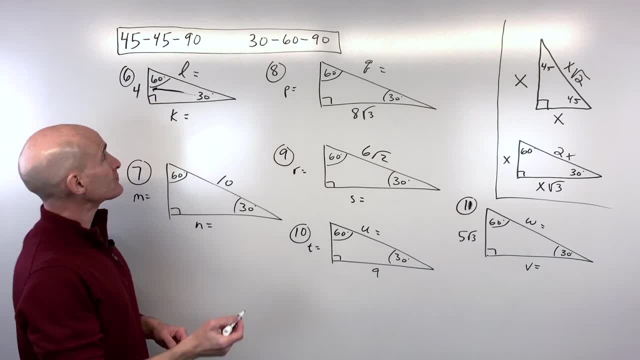 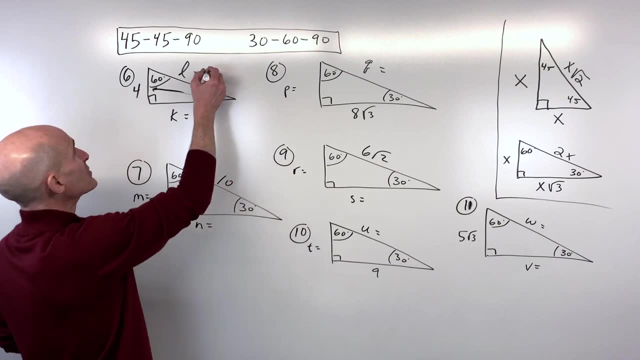 30 degree angle. that's the shortest leg, that's 4.. So if I want to get to this side here, the hypotenuse- all I have to do is double it. see x- 2x. so if I multiply by 2, I get 8, and if I want to get 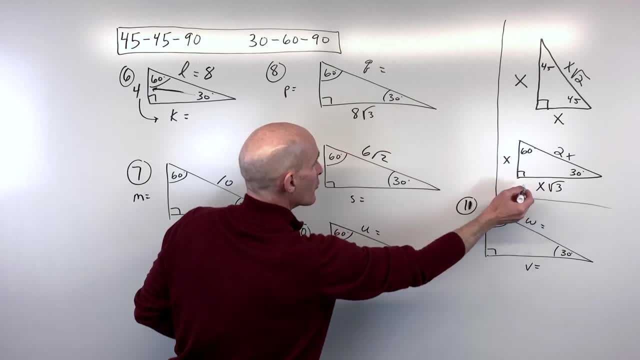 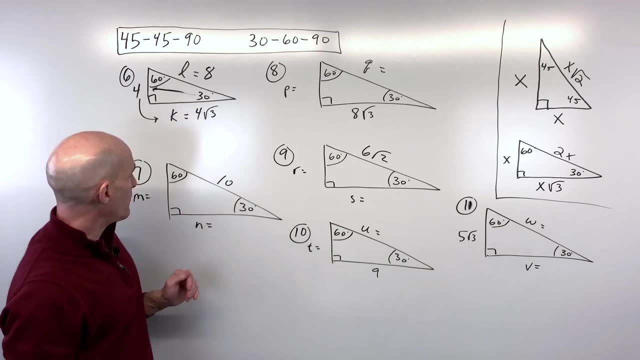 to this longer leg. I just take the shorter leg and I multiply by square root of 3, so this is going to be 4 square root of 3.. Pretty easy, right? So let's try number seven. so this one. what are they giving us? they're giving us a side across from the right angle. that's our hypotenuse and we can see that's. 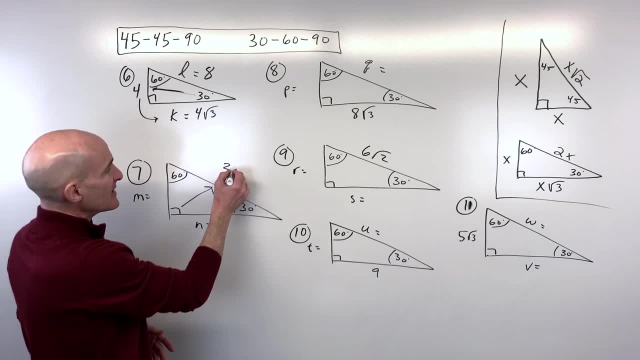 our hypotenuse and we're going to multiply by square root of 3. we're going to multiply by square root of 3 and we're going to get that side. Now, sometimes what students do to kind of help themselves out a little bit is they might kind of like superimpose these variables over the triangles. They might say: 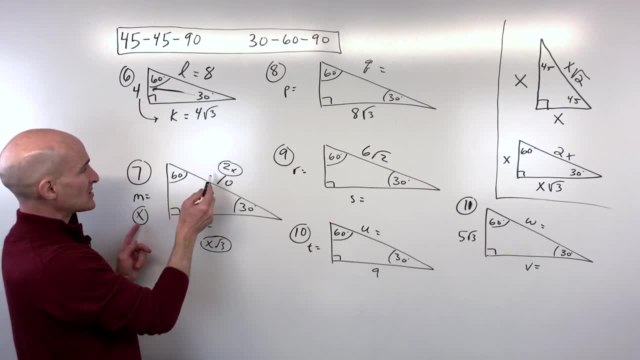 oh, that's my 2x side, this is like my 1x side, this is my like x root 3 side. So then you would say: well, hmm, how do I go from 2x to 1x? Well, I'd have to divide by 2 to get 1x. so if I take 10, 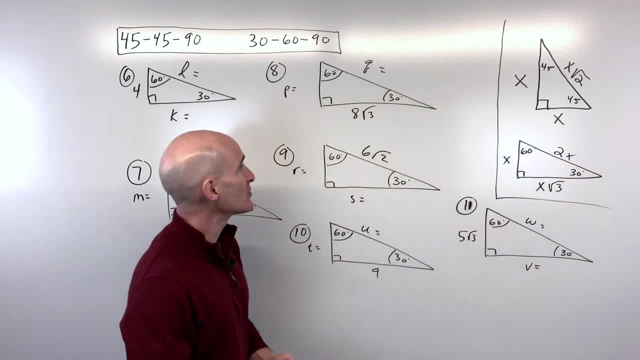 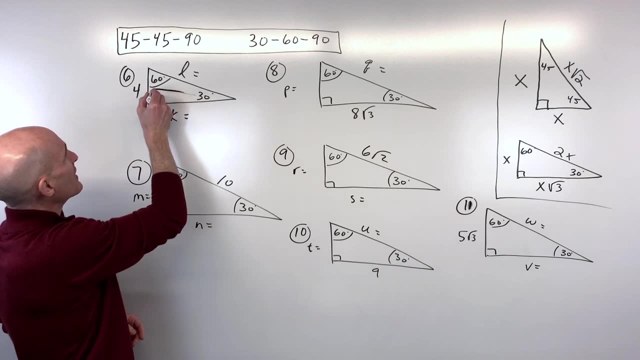 and then double it to get the hypotenuse. So let's go through some examples so you can see how this works and I'll kind of explain as I go. So for number six, you can see that they're giving us a cross from that 30 degree angle. That's the shortest leg, that's 4.. So if I want to get to this side here, 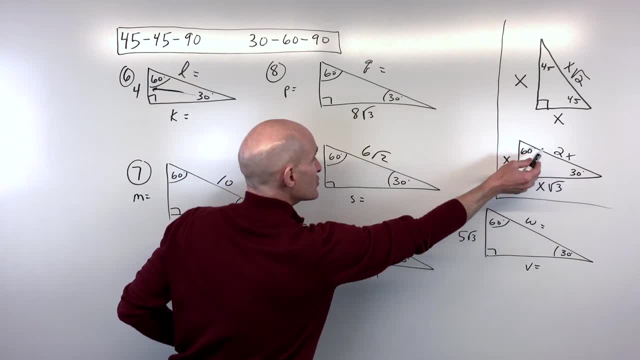 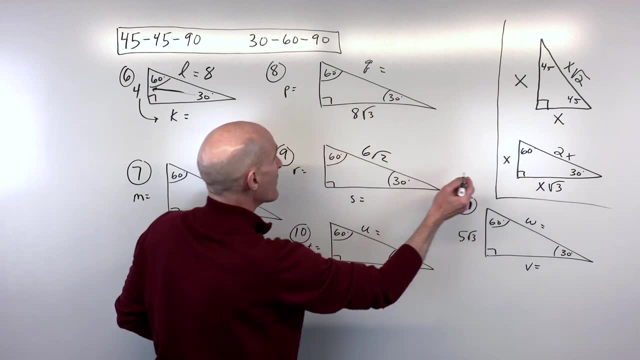 the hypotenuse. all I have to do is double it, See x- 2x. So if I multiply by 2, I get 8. And if I want to get to this longer leg, I just take the shorter leg and I multiply by square. 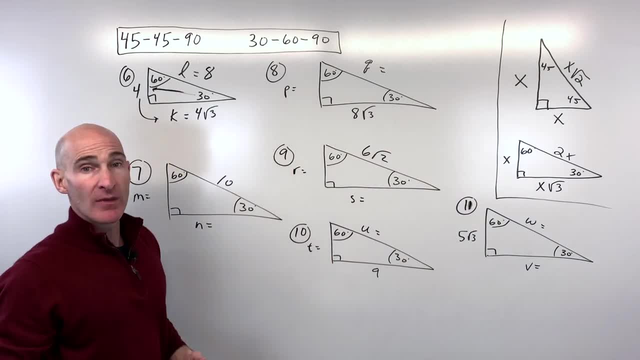 root of 3.. So this is going to be 4 square root of 3.. Pretty easy, right? So let's try number seven. So this one. what are they giving us? They're giving us a side across from the right angle. 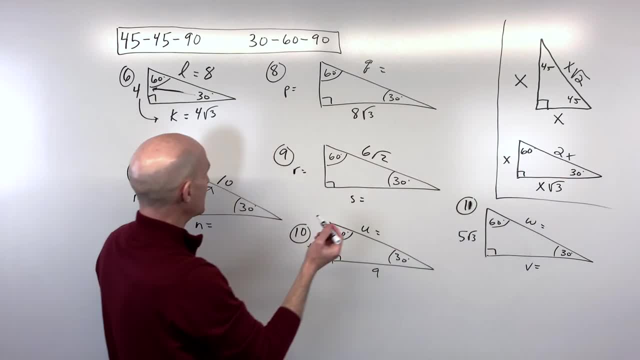 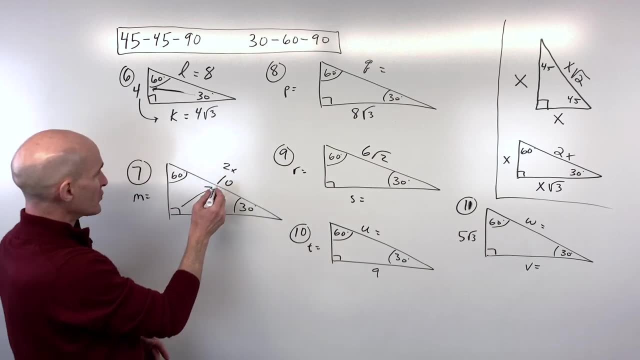 that's our hypotenuse And we can see that's the 2x side. Now sometimes what students do to kind of help themselves out a little bit is they might kind of like superimpose these variables over the triangles. They might say: oh, that's my 2x side. 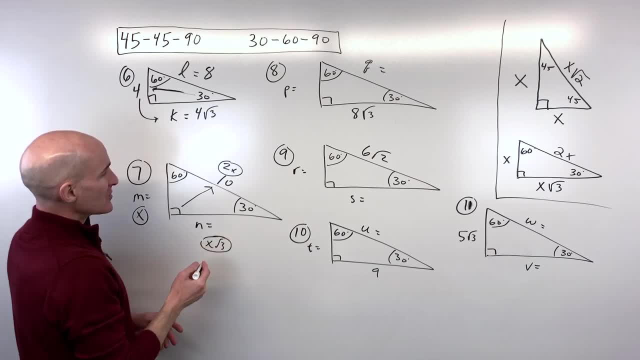 this is like my 1x side, this is my like x root 3 side. So then you would say: well, hmm, how do I go from 2x to 1x? Well, I'd have to divide by 2 to get 1x. So if I take 10 divided by 2, I get 5.. And then 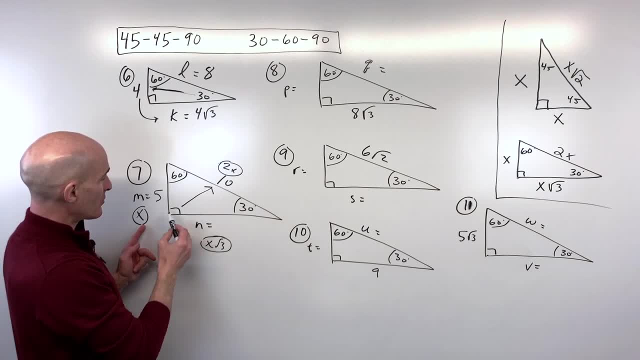 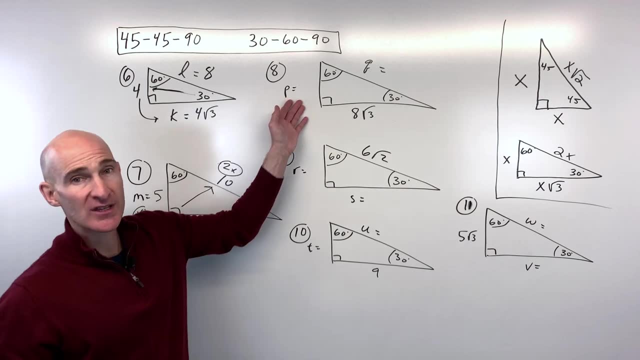 if I say: well, how do I get from x to x, root 3?? Well, I have to multiply by square root of 3.. So 5 to 3.. So that can sometimes help. After doing it a while, you just kind of know what to do. So 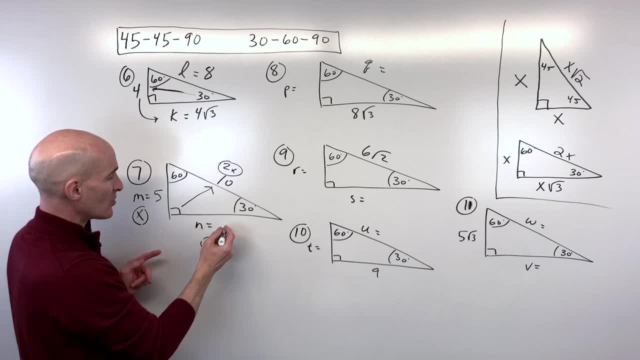 divided by 2, I get 5. and then if I say: well, how do I get from x to x root 3?? Well, I have to multiply square root of 3.. So that can sometimes help. After doing it a while, you just kind. 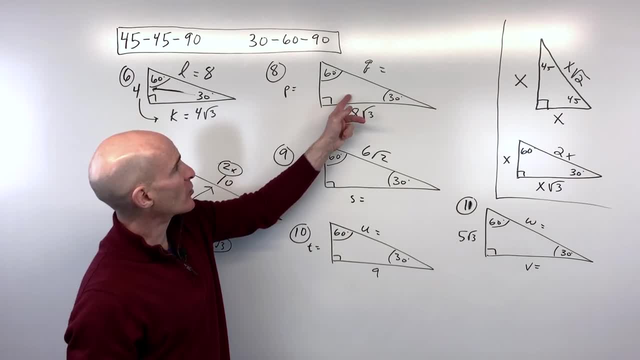 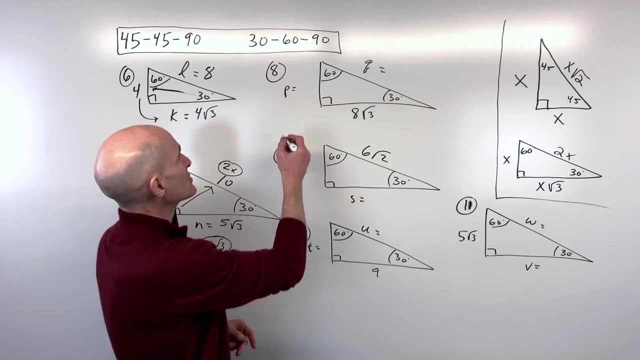 of know what to do. So, for example, this one, they're giving us the one across from the 60 degree angle, That's our longer leg, That's our x root, 3 side. So we're going to divide by the square root of 3.. So this is going to be 8 square root of 3. 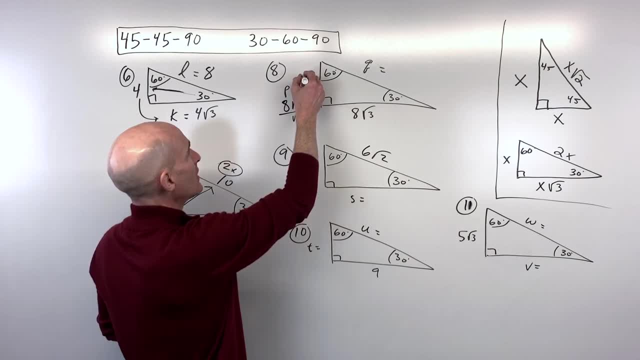 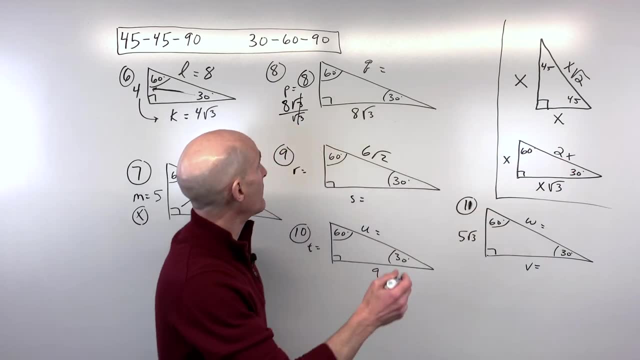 divided by square root of 3.. The square root of 3's cancel and you can see we're just getting 8.. Once you have the short leg that's pretty easy, because you just have to then double it to get the hypotenuse. So 8 double is going to give. 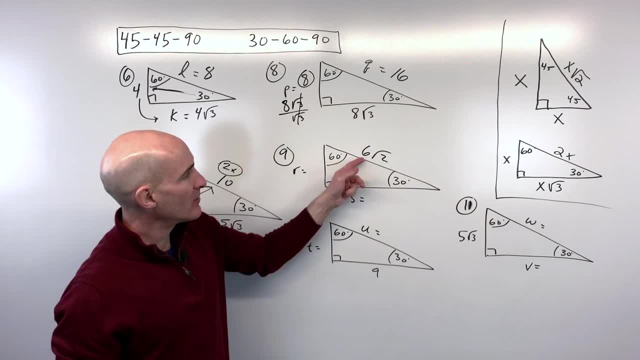 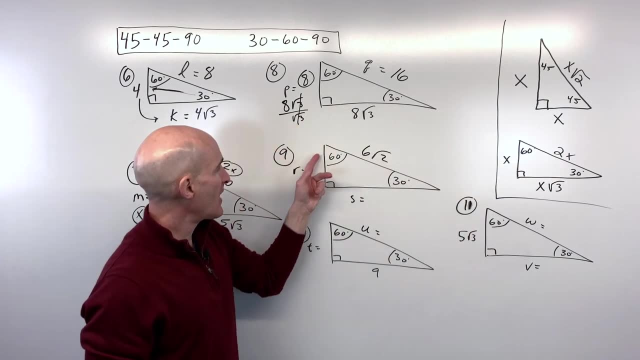 us 16.. Okay for number 9, now a little bit more challenging. They're giving us the hypotenuse, the one across from the right angle. That's our 2x side. We want to make our way back to the short leg, the 1x side, across from the 30 degree. 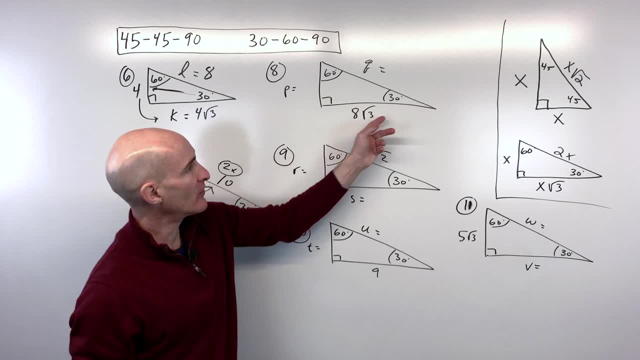 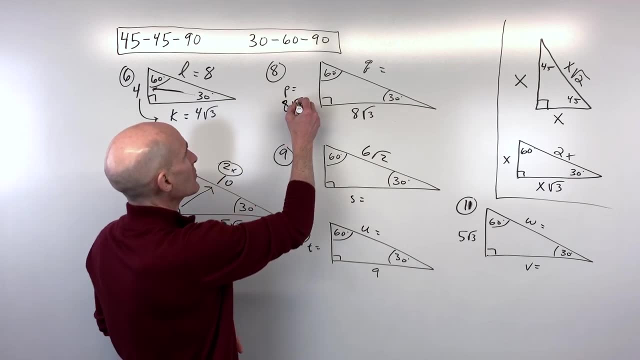 for example, this one they're giving us, the one across from the 60 degree angle, that's our longer leg, that's our x root 3 side. So we're going to divide by the square root of 3.. So this is going to be 8 square root of 3 divided by square root of 3.. The square root of 3's cancel. 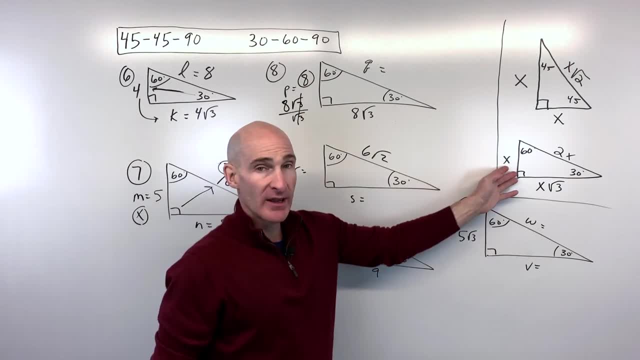 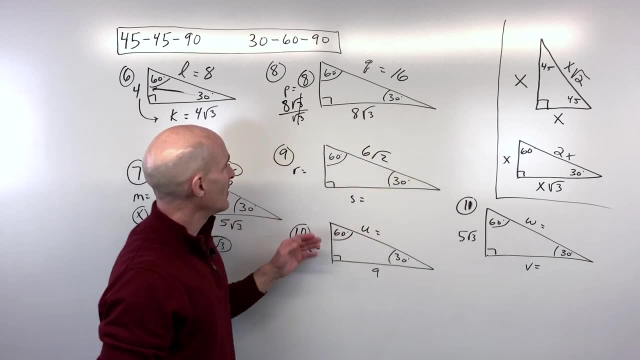 and you can see we're just getting 8.. Once you have the short leg, that's pretty easy, because you just have to then double it to get the hypotenuse. So 8 double is going to give us 16.. Okay for number 9, now a little bit more challenging. they're giving us the hypotenuse. 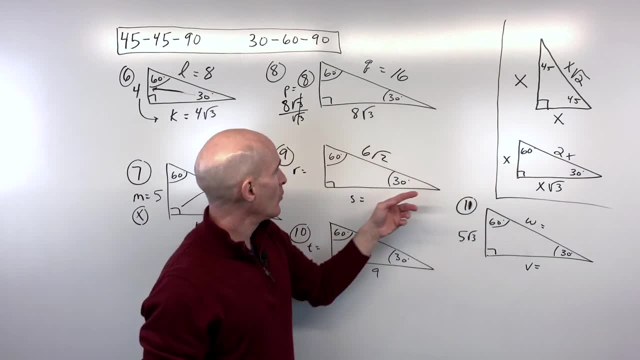 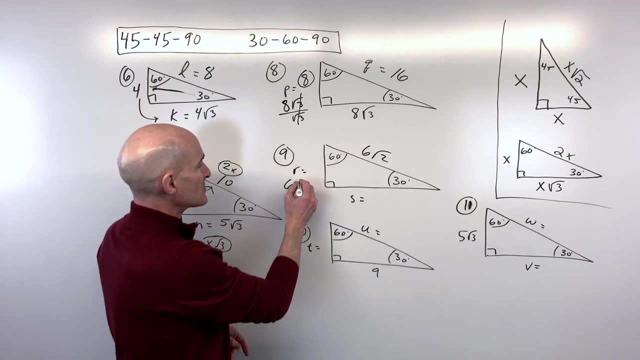 the one across from the right angle. That's our 2x side. We want to make our way back to the short leg, the 1x side, across from the 30 degree angle, which means we have to divide by 2.. So this is 6. 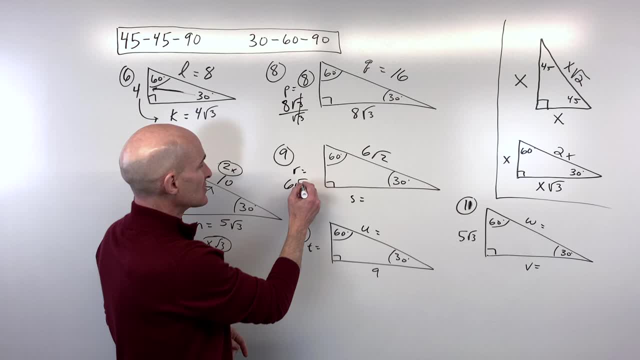 angle, which means we have to divide by 2.. So this is 6 square root of 2 divided by 2.. The 6 and the 2 reduce, So this is just going to come out to 3 root 2.. Now 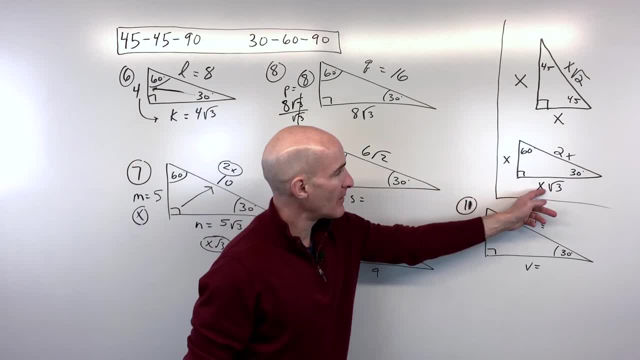 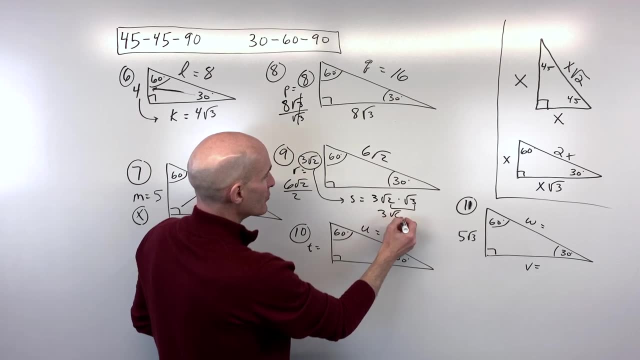 we want to make our way to the longer leg. We do that by multiplying by the square root of 3.. So 3 square root of 2 times square root of 3.. We multiply these radicals together and we get 3 square root. 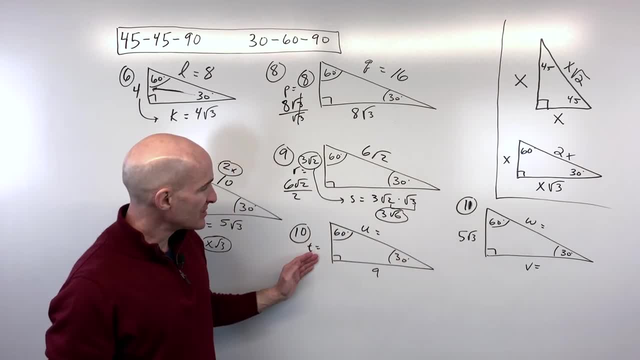 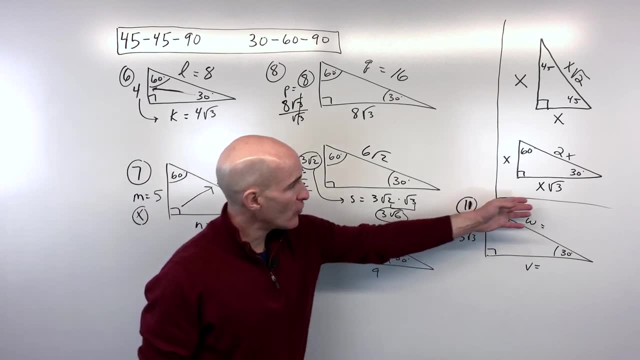 of 6 for this longer leg, Number 10,, a little bit more challenging. They're giving us the side across from the 60 degree angle. This is the longer leg, This is 9.. We want to go from that longer leg to the shorter leg and we're going to do that by dividing by the. 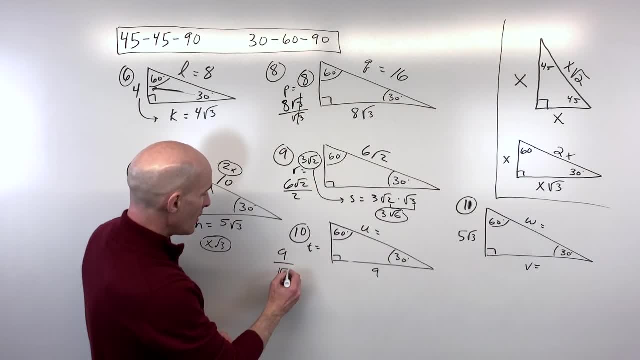 square root of 3.. So what's 9 divided by the square root of 3?? Well, we don't want that square root in the denominator, right? So we're going to rationalize by multiplying the numerator and denominator by square root of 3.. 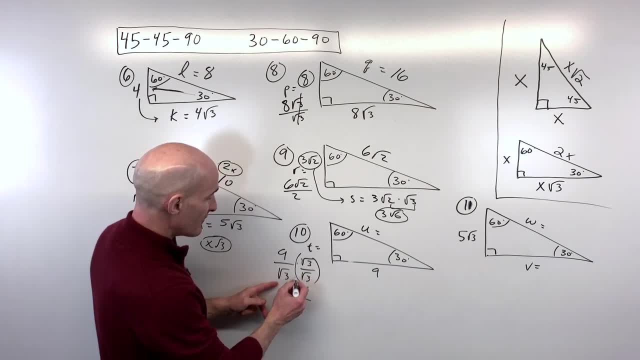 That's going to give us 9 square root of 3 over square root of 9, which is just 3.. And then the 9 and the 3 reduce, So this is just going to come out to 3 square root of 3.. 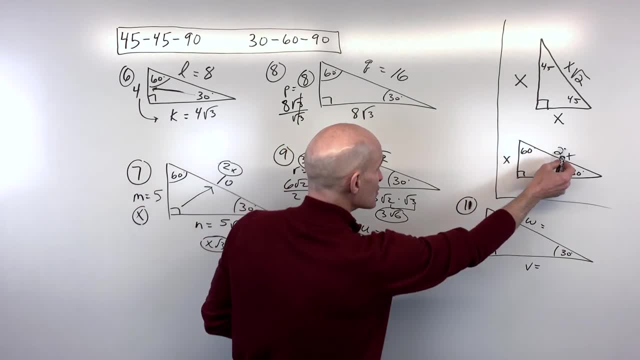 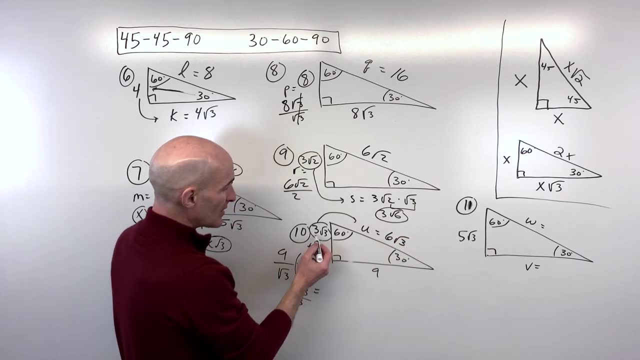 Okay now if we want to go to the hypotenuse, remember the hypotenuse is just twice the short leg. So if we multiply 3 root 3 times 2,, we get 6 square root of 3.. Don't make the. 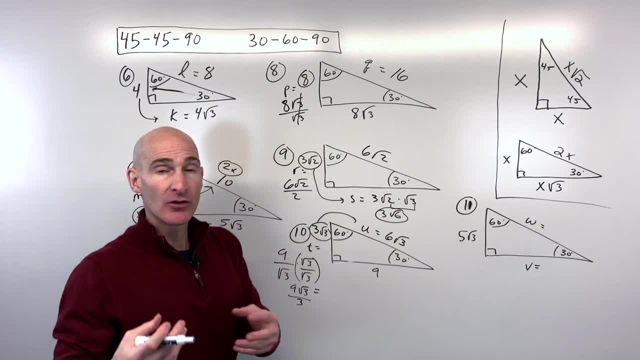 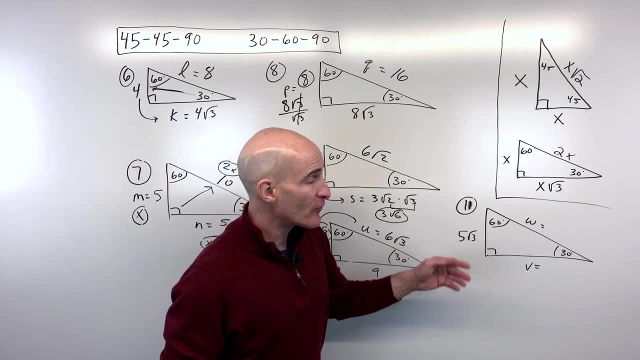 mistake of saying 6 square root of 6.. You just want to multiply the coefficients, the numbers in front together, and then you would multiply the square roots together. So it's just multiplying like terms. And our last example before we get into some more deeper explanation about the theory behind. 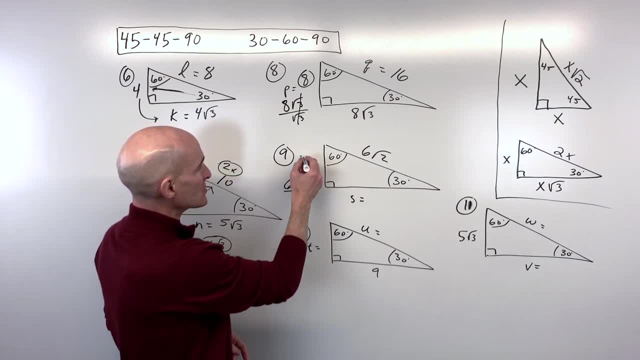 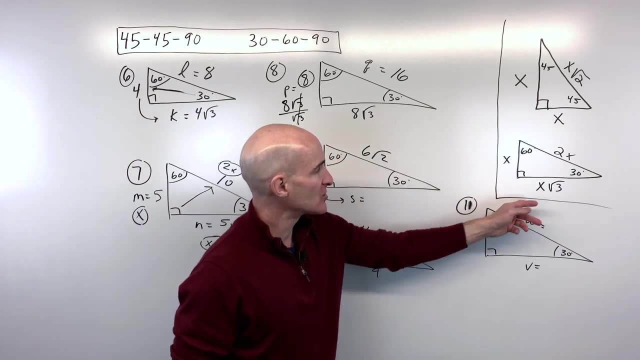 square root of 2 divided by 2.. The 6 and the 2 reduce, So this is just going to come out to 3 root 2.. Now we want to make our way to the longer leg. We do that by multiplying by the square root. 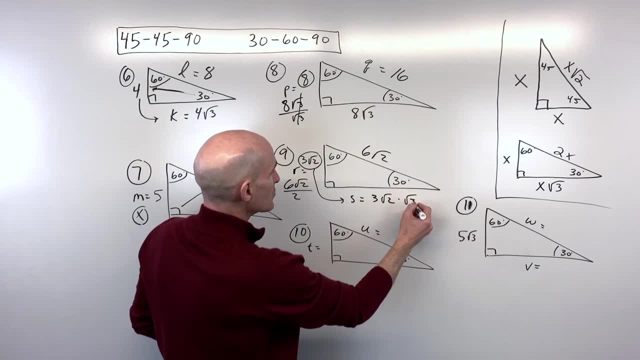 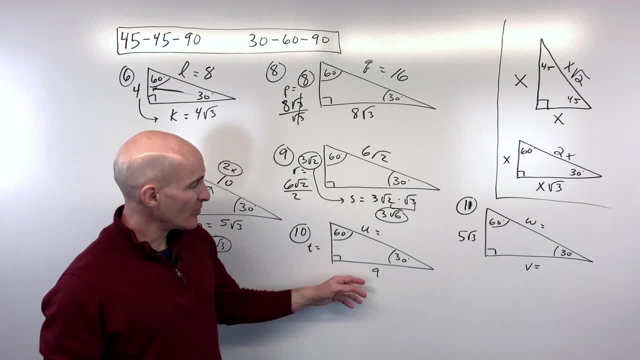 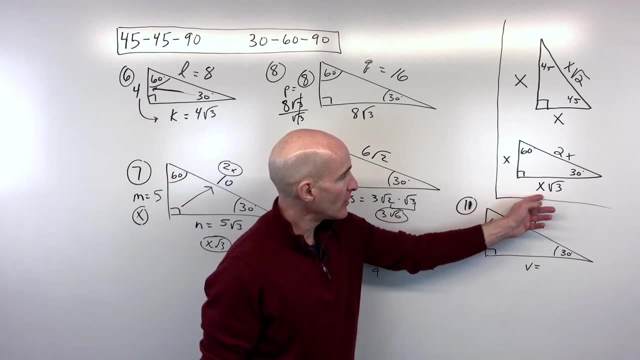 longer leg. Number 10, a little bit more challenging. they're giving us the side across from the 60 degree angle. This is the longer leg, This is 9.. We want to go from that longer leg to the shorter leg and we're going to do that by dividing by the square root of 3.. So what's 9? 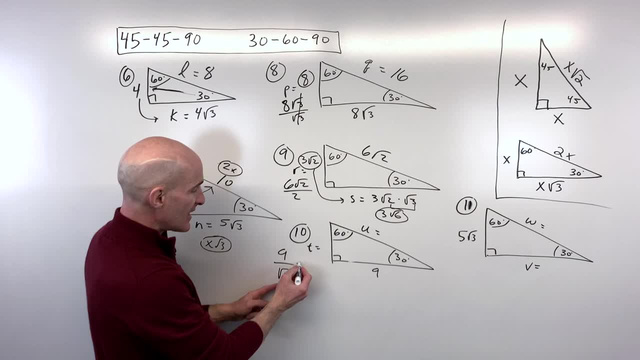 divided by the square root of 3? Well, we don't want that squared in the denominator, right? so we're going to rationalize by multiplying the numerator and denominator by square root of 3.. So that's going to give us 9 square root of 3 over square root of 9, which is just 3.. And then 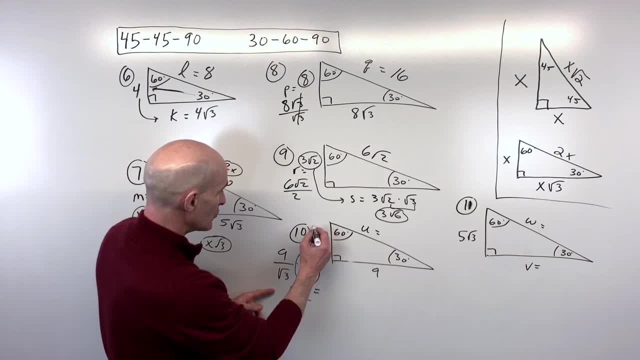 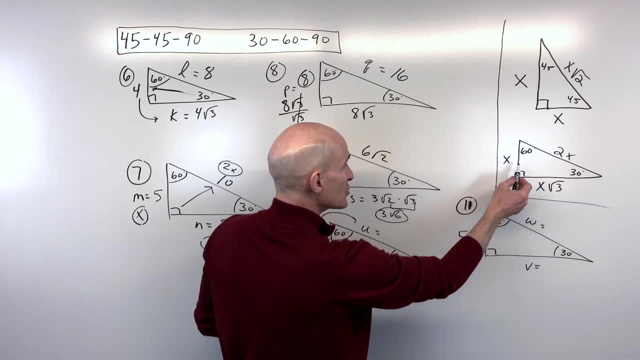 the 9 and the 3 reduce, So this is just going to come out to 3 square root of 3.. Okay now if we want to go to the hypotenuse, remember the hypotenuse is just twice the short leg. So if we multiply 3, 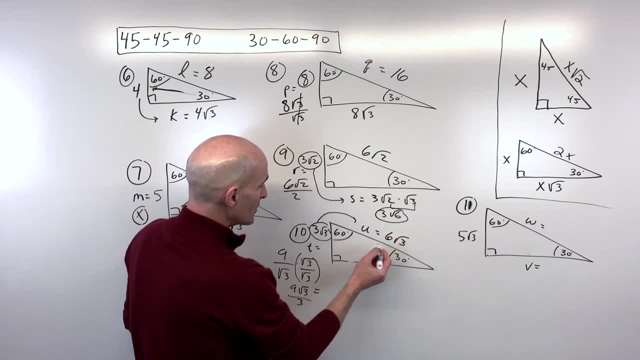 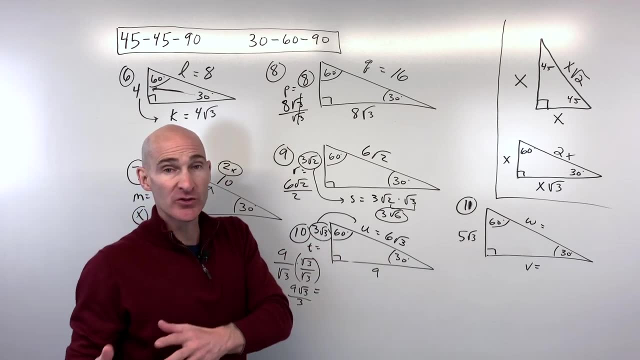 root 3 times 2, we get 6 square root of 3.. Don't make the mistake of saying 6 square root of 6, you just want to multiply the coefficients, the numbers in front, together, and then you'd multiply the roots together. So it's like multiplying like terms. And our last example, before we get into 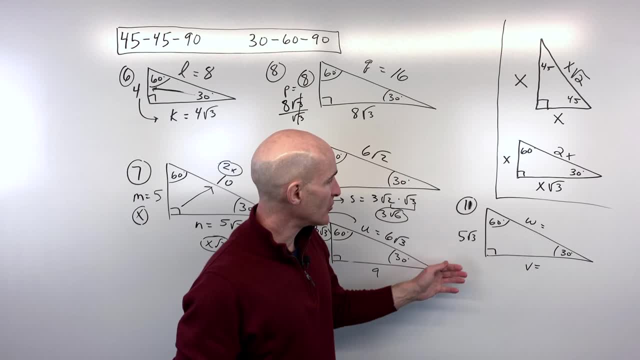 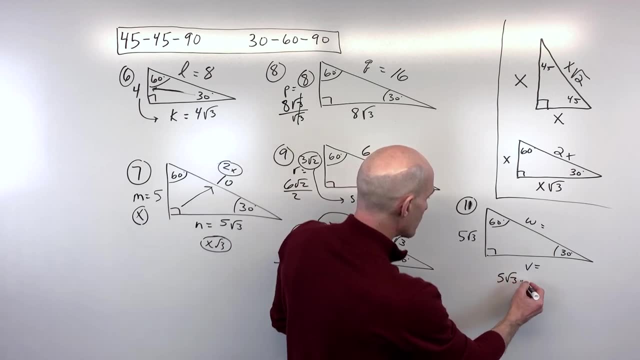 some more deeper explanation about the theory behind these two triangles. Here. they're giving us the shorter leg and what we want to do is we want to go to the longer leg, So we have to multiply by the square root of 3.. Square root of 3 times square root of 3 is square root of 9,. 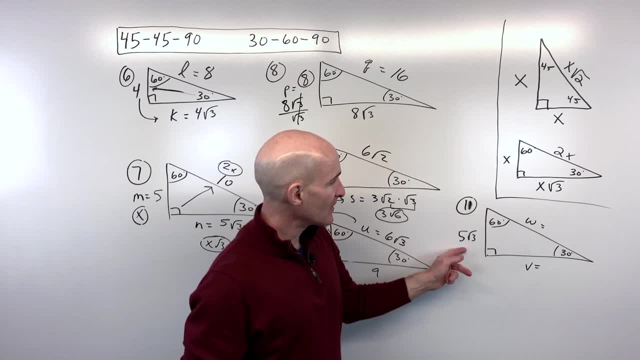 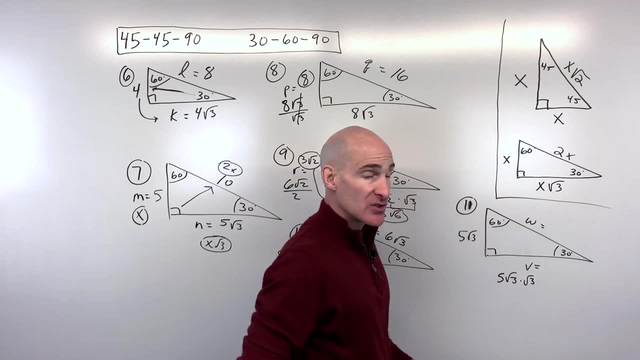 these two triangles here. they're giving us the shorter leg and what we want to do is we want to go to the longer leg. So we have to multiply by the square root of 3.. Square root of 3 times square root of 3 is square root of 9, which is just 3, times this 5 is. 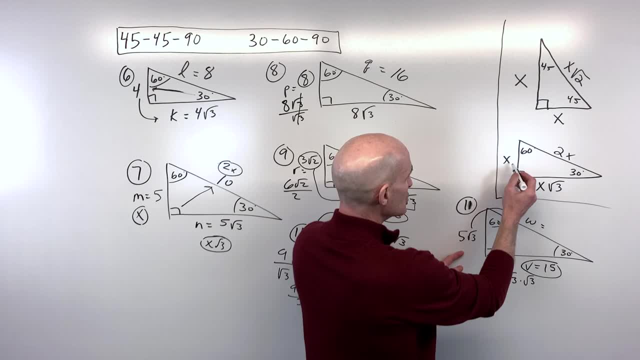 going to give us 15.. And if we want to go to the hypotenuse, we just have to double that shorter leg and 5 root 3 times 2 is going to give us 10 square roots of 3.. Again, remember. when we multiply by 2, we're going to multiply by 10 square roots of 3.. So we're going to multiply by 10 square roots of 3.. Again, remember, when we multiply by 2, we're going to multiply by 10 square roots of 3.. Again, remember when we multiply by 10 square roots of 3.. So we're. 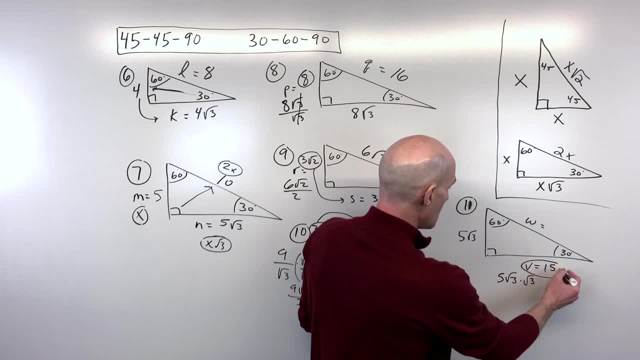 which is just 3 times this. 5 is going to give us 15.. And if we want to go to the hypotenuse we just have to double that shorter leg and 5 root 3 times 2 is going to give us 10 square. 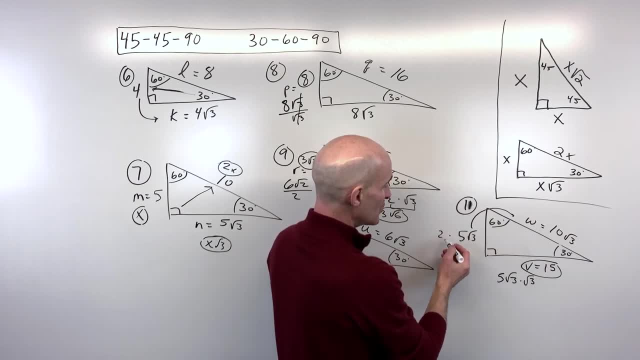 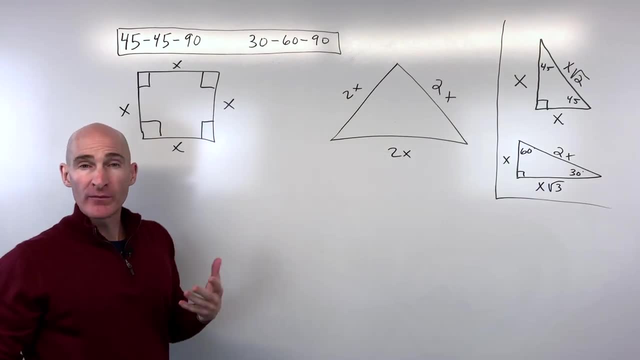 roots of 3.. Remember, when we multiply by 2, we're just multiplying those integers together and not. you know, there's no square root, so the square root just comes along with it. Okay, for those of you that want to know a little bit more about you know why this works and where these 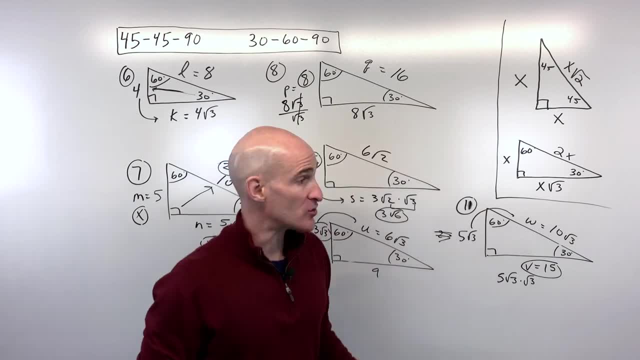 going to multiply by 10 square roots of 3.. So we're going to multiply by 10 square roots of 3.. And again, what we're going to do, we're just multiplying those integers together and not. you know, there's no square root, so the square root just comes along with it. 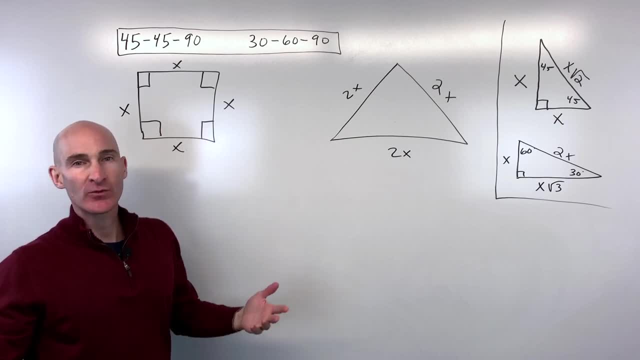 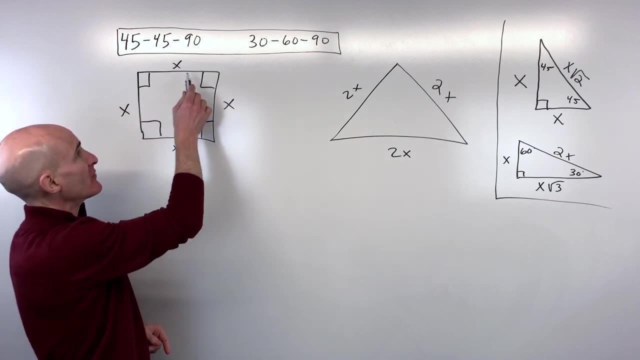 Okay, for those of you that want to know a little bit more about you know why this works and where these values come from. let's start off by looking at a square. Now we know in a square you've got these four right angles and you have these four congruent sides. We're 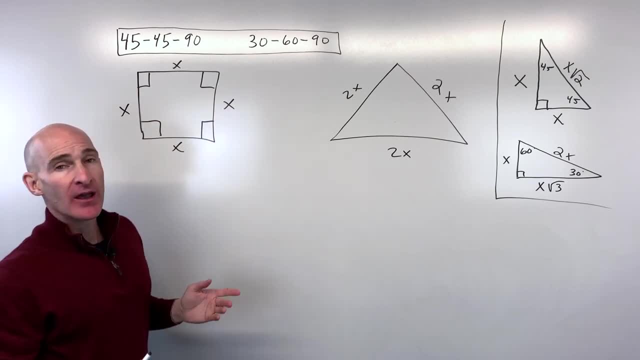 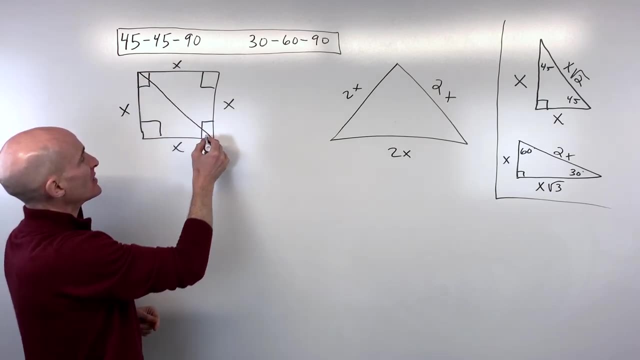 going to call each of the sides x, because they're all the same, right. But what we're going to do now is we're going to draw a diagonal like so, And we're going to look at this triangle. No diagonal that's going to bisect this angle here. This is going to be a 45-45-90 triangle and it's 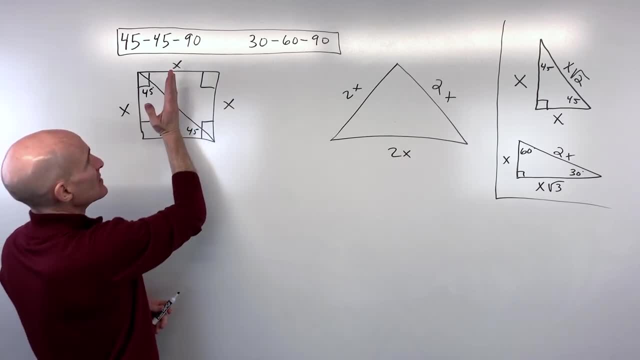 kind of like, if you're trying to put something in a box, Like, if you try to put it this way, sometimes it doesn't fit. If you try to put it this way, it doesn't fit, What do we naturally do? We put it on the diagonal, because we know that diagonal is going to be longer and in fact we 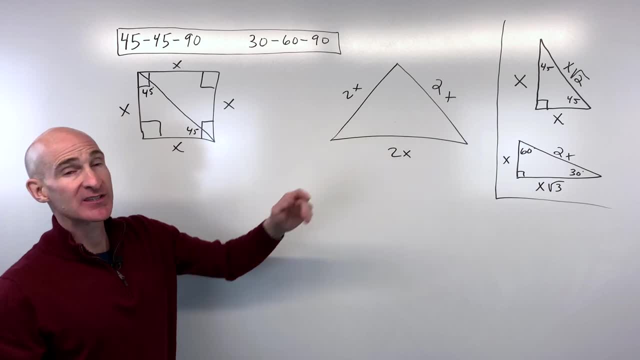 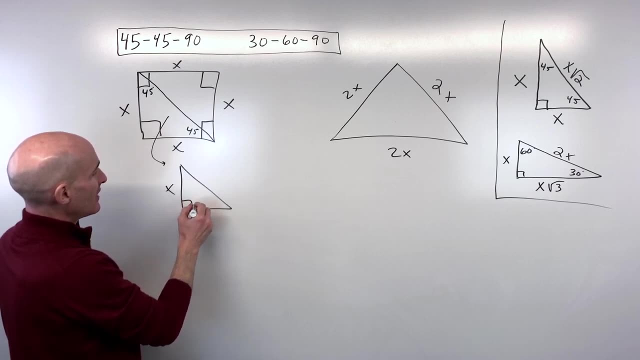 know it's about 1.4 times longer, or square to two times longer, But let's see if we can understand why that is So. if we take this triangle now, let's draw it here, We've got x, x and let's call. 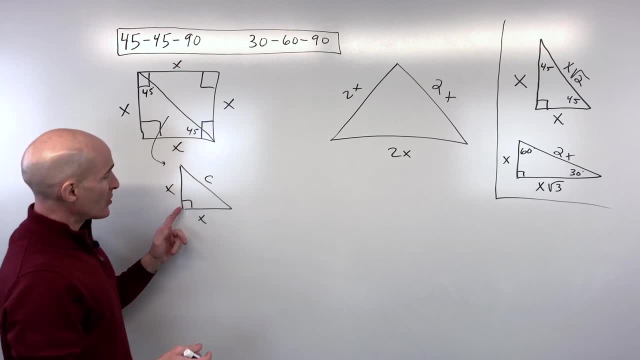 this side c. Now you remember your Pythagorean theorem: a squared plus b squared equals c squared right. So the sum of the two legs squared equals the hypotenuse squared. So let's go ahead and write that formula down. So a squared plus b squared equals c squared. Here this is going to: 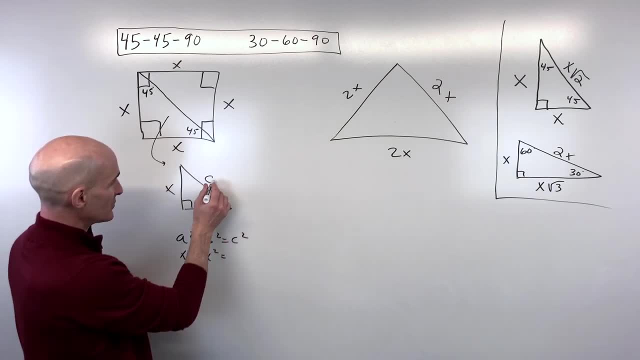 be x squared plus x squared is equal to this hypotenuse squared. This comes out to 2x squared equals c squared And if we take the square root just to get the length of c, the square root of x squared is going to be x squared to two. We're just going to. we can't really simplify that, we'll just leave it. 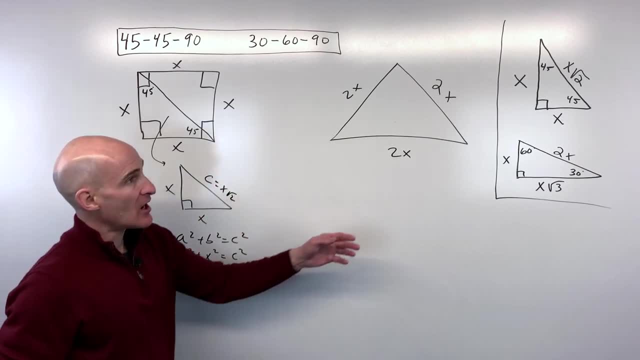 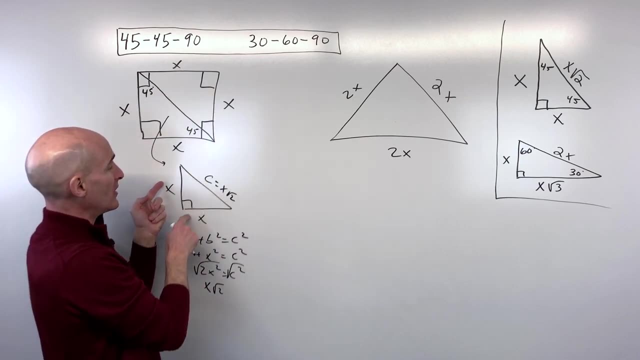 as square root of two. So that's where these values are coming from for the 45, 45, 90.. The two legs are the same, Remember, because this is coming from the square where all the sides are congruent, but the hypotenuse is x squared to two, and that comes from our Pythagorean theorem. 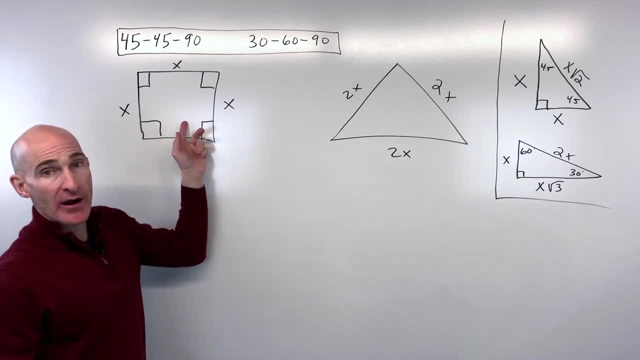 values come from. let's start off by looking at a square. Now, we know in a square you've got these four right angles and you have these four congruent sides. We're going to call each of the sides x, because they're all the same right, But what we're going to do now is we're going to draw a diagonal. 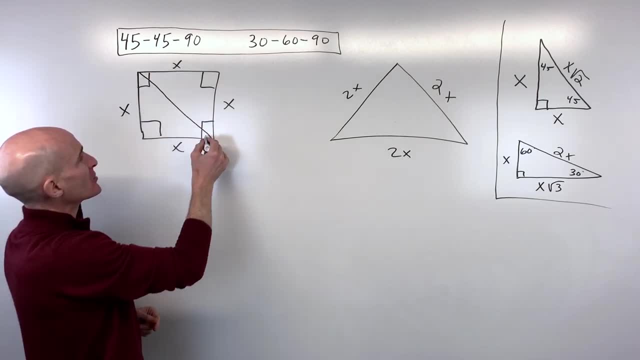 like so, And we're going to look at this triangle now when we draw a diagonal that's going to bisect this angle here. This is going to be a 45-45-90 triangle And it's kind of like if you're trying to put something in a box, Like if you try to put 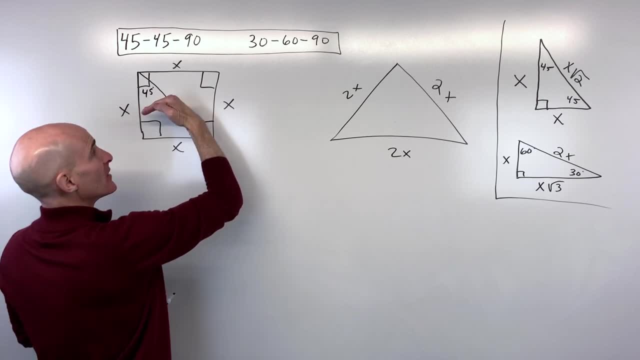 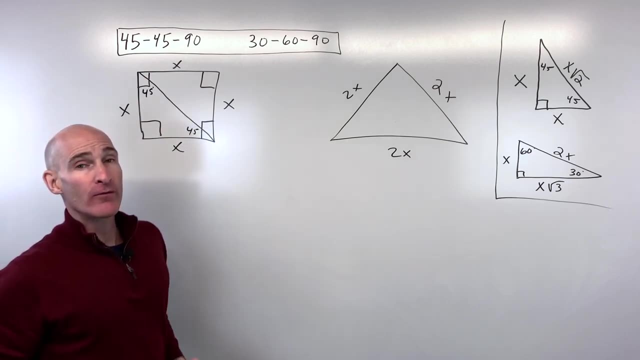 it this way. sometimes it doesn't fit. If you try to put it this way, it doesn't fit. What do we naturally do? We put it on the diagonal because we know that diagonal is going to be longer and in fact we know it's about 1.4 times longer, or square root of 2 times longer. But let's see. 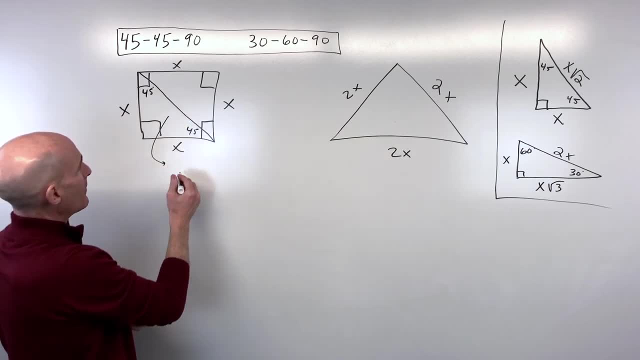 if we can understand why that is So. if we take this triangle, now let's draw it here. We've got x and let's call this side c. Now you remember your Pythagorean theorem: a squared plus b squared equals c squared right. So the sum of the two legs squared equals the hypotenuse squared. So let's go. 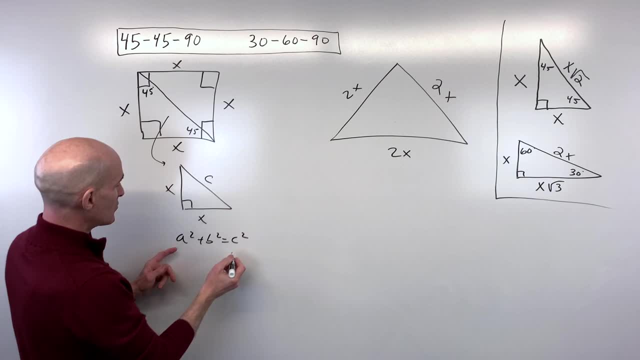 ahead and write that formula down. So a squared plus b squared equals c squared. Here this is going to be: x squared plus x squared is equal to this hypotenuse squared. This comes out to: 2x squared equals c squared, And if we take the square root just to get the length of c, the 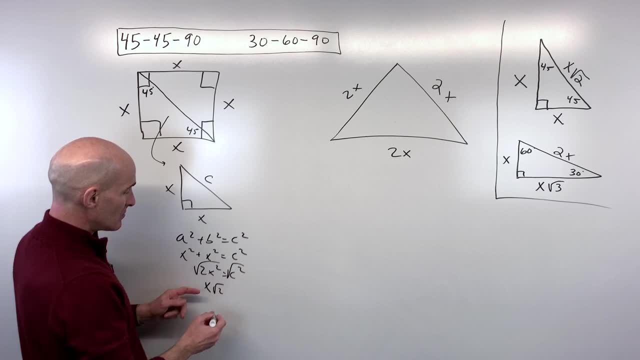 square root of x. squared is going to be x Square root of 2, we're going to get the length of c. We can't really simplify that. We'll just leave it as square root of 2.. So that's where these values 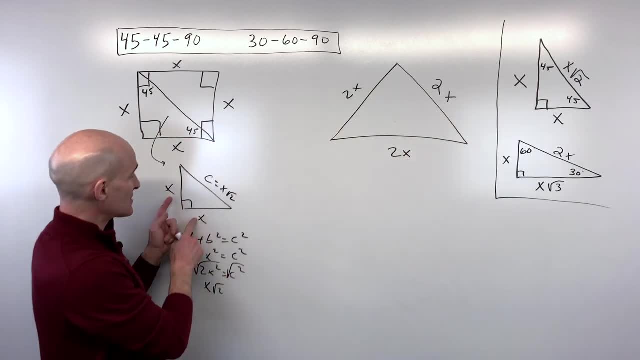 are coming from for the 45-45-90.. The two legs are the same, Remember, because this is coming from the square where all the sides are congruent, But the hypotenuse is x squared to 2, and that comes from our Pythagorean theorem. Now let's jump over to the 30-60-90.. Now we're going to start with an. 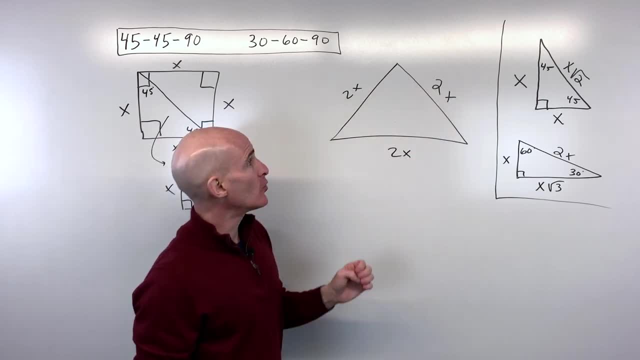 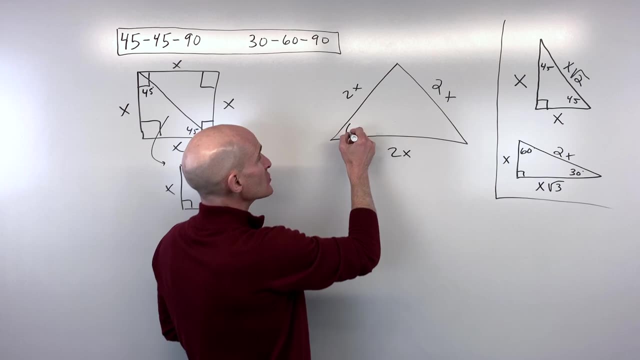 equilateral triangle. Now, remember, lateral means side, equal means equal. But if it's equilateral and all the angles in a triangle add up to 180, so if all these angles are equal, they must all be 60 degrees. right Now, if we drop an altitude, okay, in an isosceles triangle, an equilateral 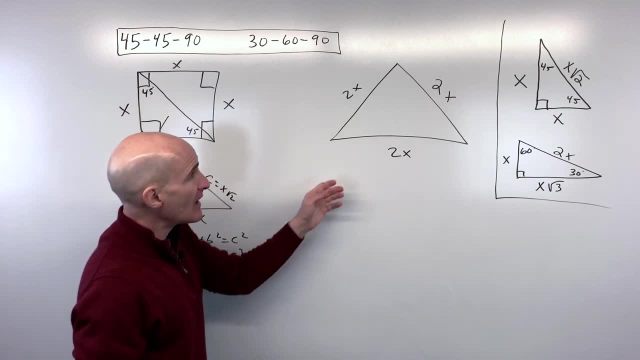 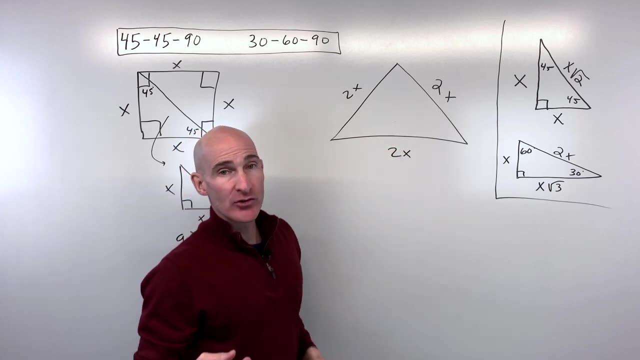 Now let's jump over to the 30, 60, 90. Now we're going to start with an equilateral triangle. Now remember, lateral means side, equa means equal. But if it's equilateral, we also know it's equiangular and all. 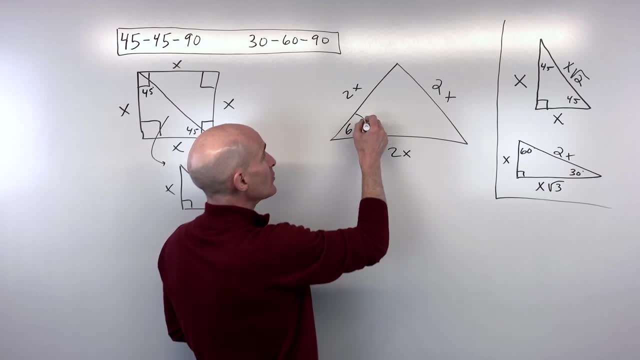 the angles in a triangle add up to 180. So if all these angles are equal, they must all be 60 degrees. right Now, if we drop an altitude- okay, in an isosceles triangle- an equilateral triangle is a special type of isosceles triangle- what happens is it's going to be perpendicular to the base. 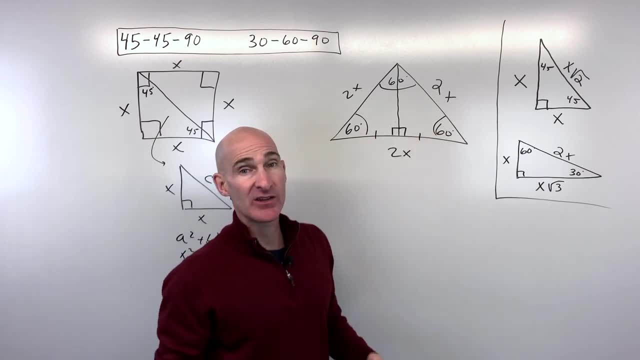 meaning it forms a right angle, and it's also going to bisect the base, meaning it's going to cut it in half. So if this whole length is 2x, now, this is going to be perpendicular to the base, meaning it's going to be at 60 degrees, which is a right angle. now this is going to be x and this is going to be x. 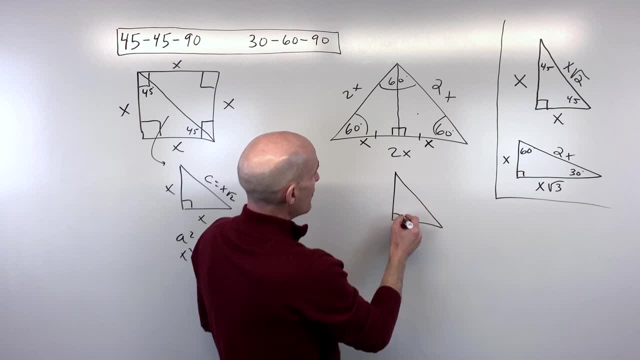 Let's take a look at this triangle right here. Let's draw it down here. So now what we're getting is we're getting x- 2x. this angle is 60 degrees and this angle is going to be 30 degrees because all the angles add up to 180. but we also know that when we drop that altitude here, it bisects this: 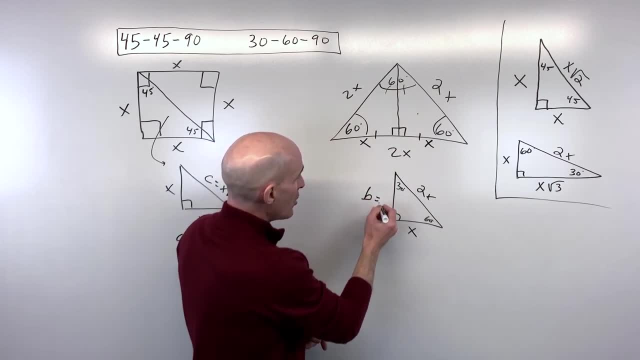 vertex angle. So now we're going to solve for the side here- Let's just call it b- and we're going to do our Pythagorean theorem again: a squared plus b squared equals c squared, solving for this leg. so we've got a squared plus b squared equals c squared. we're going to say: 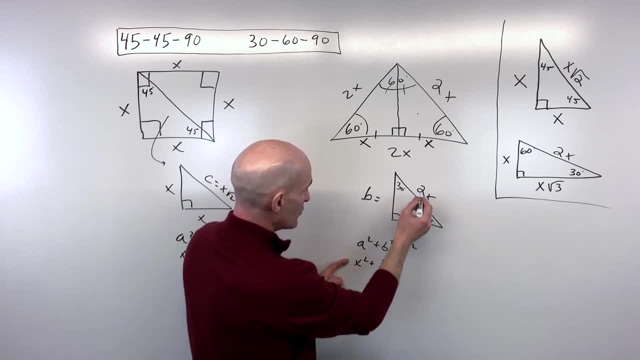 x squared plus b squared, which is a side, equals 2x. the quantity squared, right, that whole thing squared 2x times 2x is 4x squared, and if we subtract x squared from both sides, we're going to get b squared is equal to 3x squared, and if we take the square root of both sides to get b by, 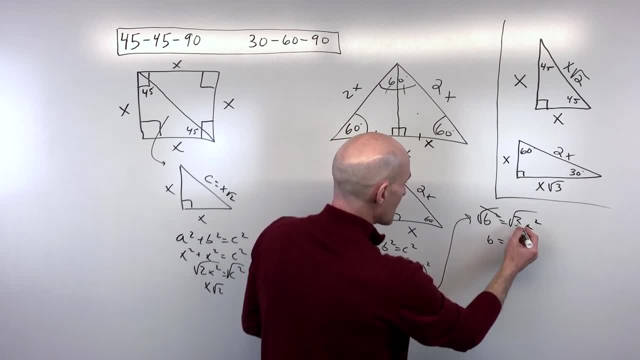 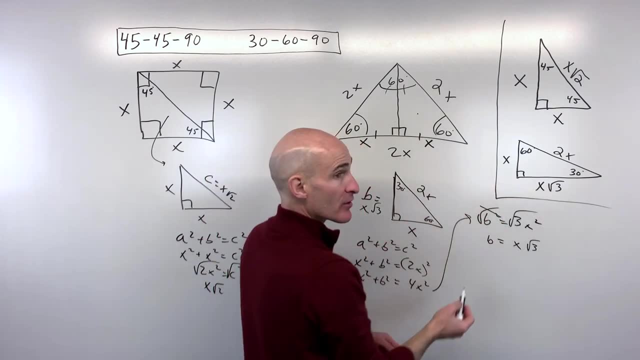 itself. you can see we're getting square root of x. squared is x and we have the square root of 3 left over. so that tells you here that our longer leg is going to be x, squared 3, the one that's across from the 60 degree angle. that's our longer leg. x root 3, one across from the 30 is the short. 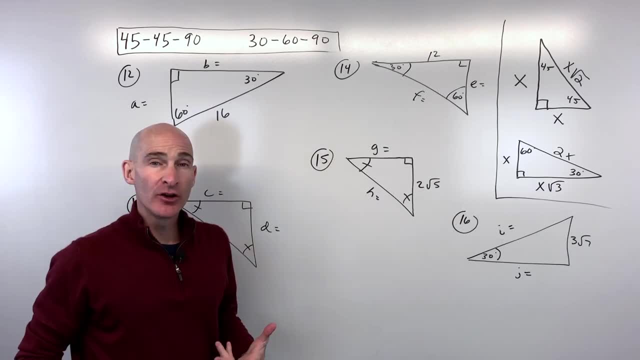 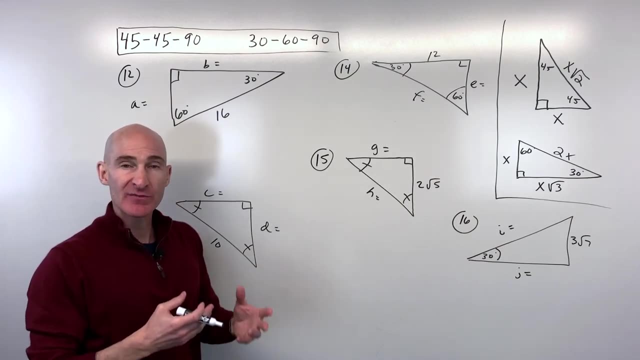 leg x and our hypotenuse is the longest one, 2x. Okay, here's a little bit of an opportunity for you to practice on your own, so what you might want to do is take a screenshot, see if you can solve these five problems. I kind of mixed them up randomly. see if you can do them and we'll go. 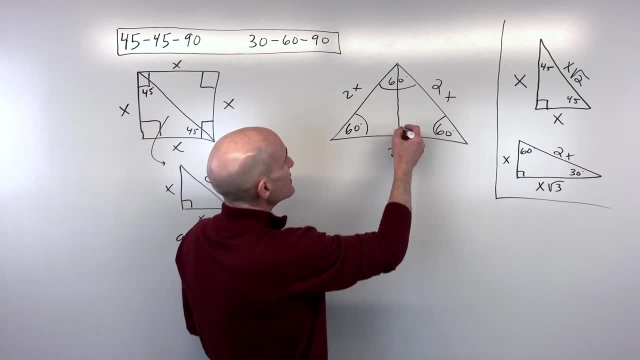 triangle is a special type of isosceles triangle. what happens is it's going to be perpendicular to the base, meaning it forms the right angle, and it's also going to bisect the base, meaning it's going to cut it in half. So if this whole length is 2x, now this is going to be x and this is going. 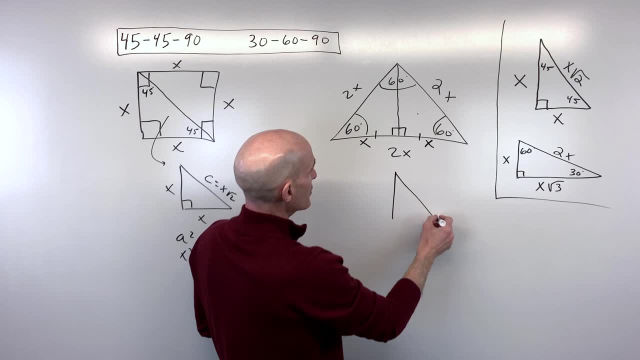 to be x. Let's take a look at this triangle right here. Let's draw it down here. So now we're getting is we're getting x, 2x. this angle is 60 degrees and this angle is going to be 30. 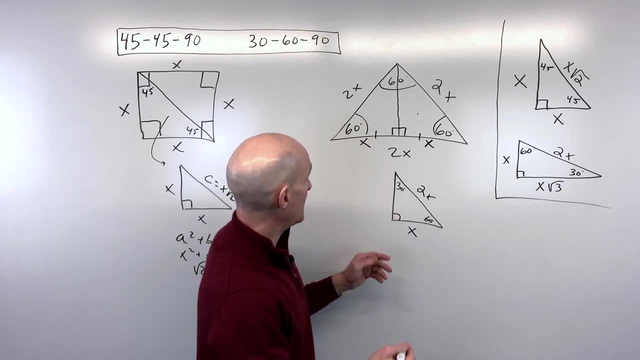 degrees, because all the angles add up to 180.. But we also know that we drop that altitude here. it bisects this vertex angle. So now we're going to solve for the side here Let's just call it b, and we're going to do our Pythagorean theorem again: a squared plus b squared equals c squared. 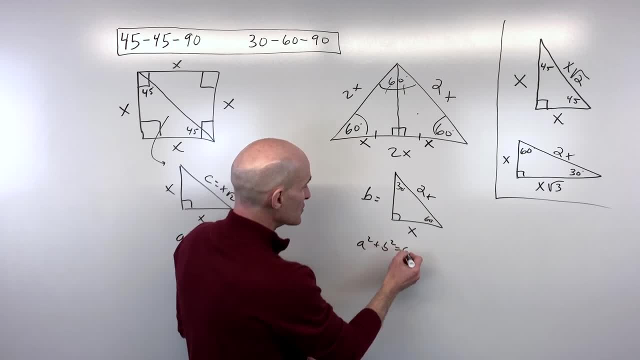 solving for this leg. So we've got a squared plus b squared equals c squared. We're going to say x squared plus b squared, which is a side, equals 2x the quantity squared. right, that whole thing squared 2x times 2x is 4x squared. And if we subtract x squared from both sides, we're going: 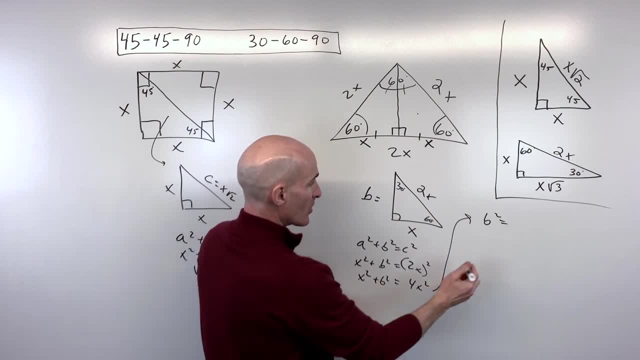 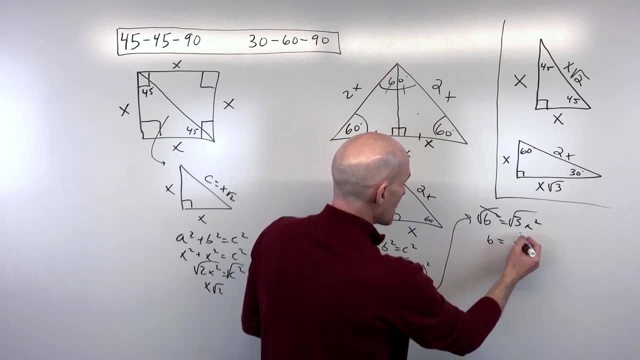 to get b squared is equal to 3x squared And if we take the square root of both sides to get b by itself, you can see we're getting square root of x squared is x and we have the square root of 3. 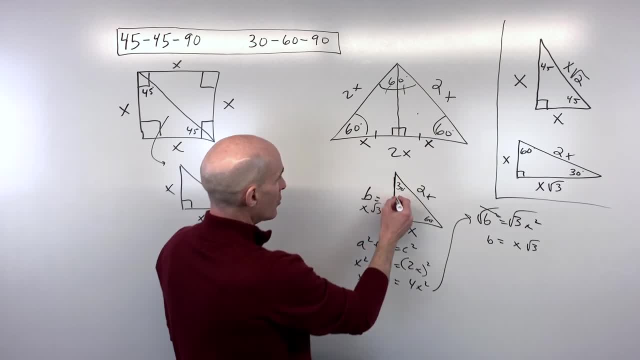 left over. So that tells you here that our longer leg is going to be a square root of x squared and our longer leg is going to be x squared of 3.. The one that's across from the 60 degree angle, that's our longer leg: x root 3.. One across from the 30 is the short leg x, and our hypotenuse is: 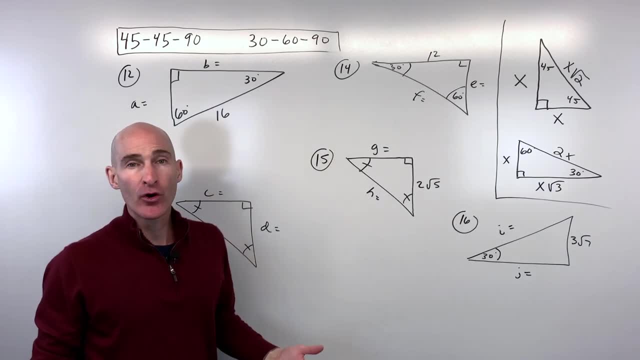 the longest one, 2x. Okay, here's a little bit of an opportunity for you to practice on your own, So what you might want to do is take a screenshot, see if you can solve these five problems. I kind of mixed them up randomly: See if you can do them, and we'll go through them together. Now for number 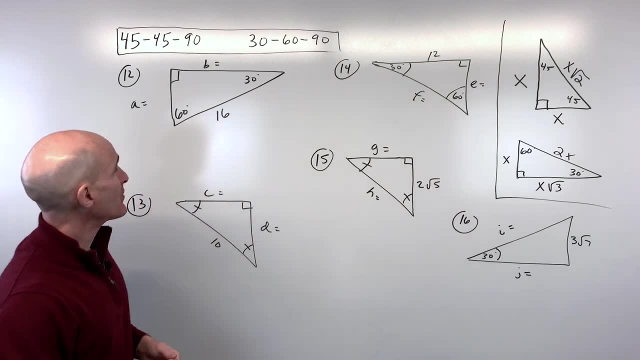 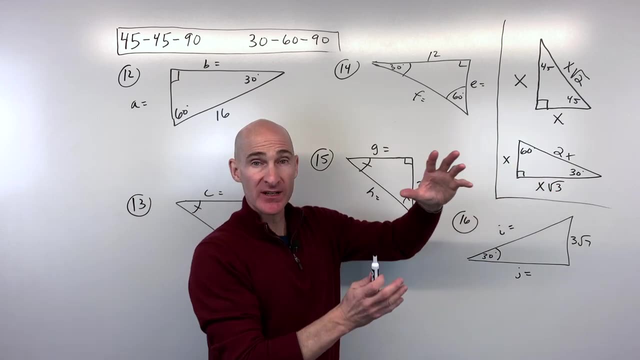 through them together. Now for number 12. if I was going to do this one on my own, one thing you'll notice is that the way that I've drawn this triangle is different than the way I explained this originally, that orientation. so I kind of rotated it, kind of changed the direction a little bit to try to make a little. 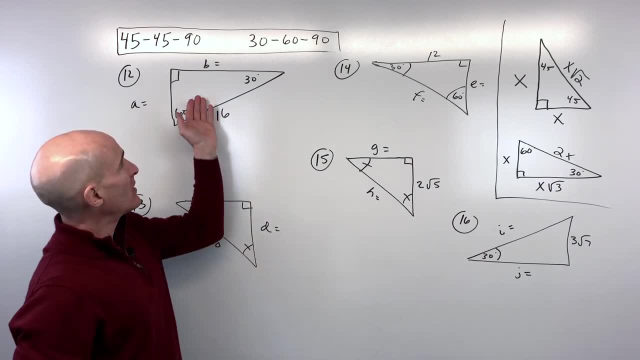 12, if I was going to do this one on my own. one thing you'll notice is that the way that I've drawn this triangle is different than the way I explained the first one, So I'm going to do this one on my own. One thing you'll notice is that the way that I've drawn this triangle is different than the. 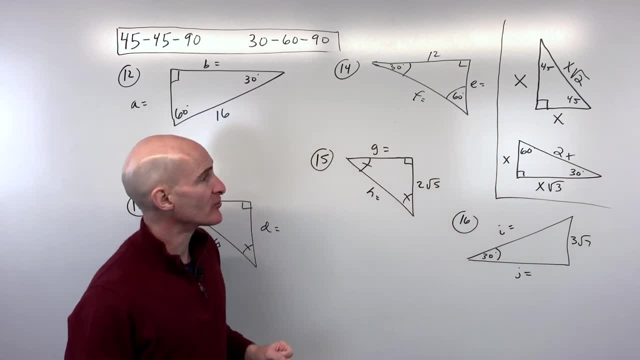 way that I've explained this originally, that orientation. So I kind of rotated it, kind of changed the direction a little bit to try to make it a little bit more challenging. Now, if you have a phone or a piece of paper, you can rotate it, so it's a little bit more familiar, a little bit more. 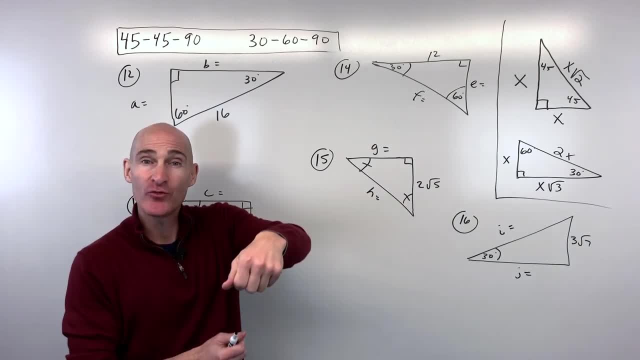 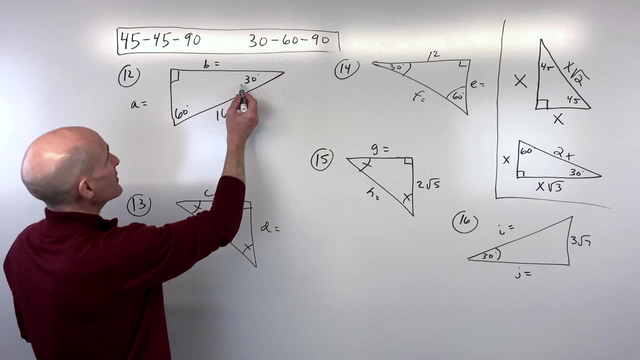 bit more challenging Now. if you have a phone or a piece of paper, you can rotate it, so it's a little bit more familiar, a little bit more comfortable if you're used to seeing it in a particular direction. but what I like to think about is, you know, short legs across from the 30 long legs. 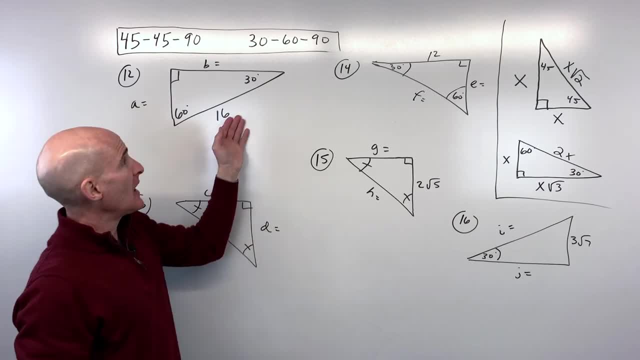 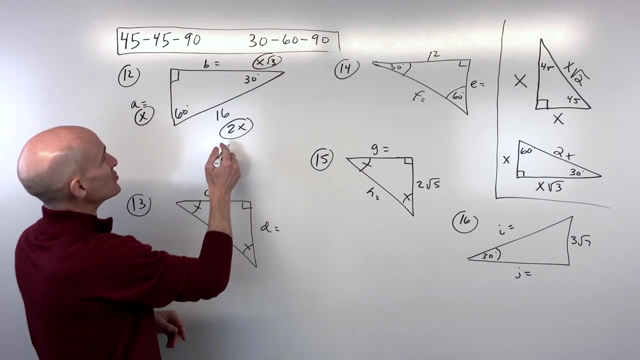 across from the 60 hypotenuse is across from the 60 long legs, across from the 60 long legs, across from the right angle, and if you want to use that little technique I was talking about earlier with the 2x, 1x and x root 3 to kind of guide you, you can say: well, hmm, they're giving us the 2x side. I 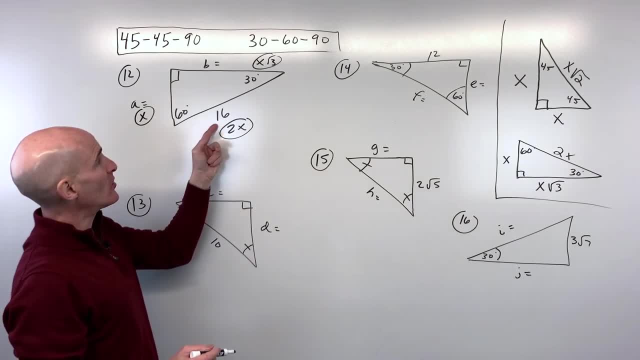 want to go back to the 1x side, so I have to divide by 2. what's 16 divided by 2? that's going to be 8. now to go from x to x, root 3. I just have to multiply by square root of 3, so 8 times square. 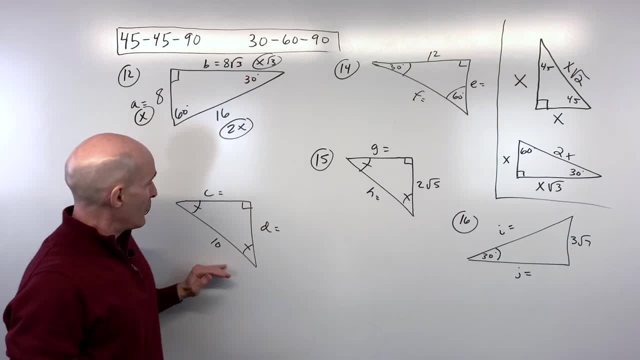 root of 3 gives us 8 square root of 3.. For number 13: this, you can see, is a 45-45-90 triangle. For number 13: this you can see is a 45-45-90 triangle. Also, I rotated it a little bit to make it a little bit more challenging and you can see they're giving. 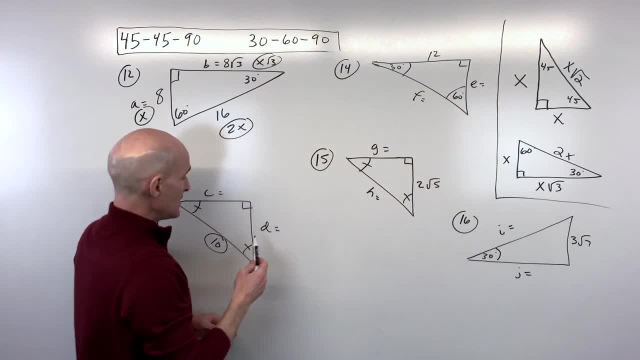 us the hypotenuse that's going to be our x root 2 side. to get back to the leg, we have to divide by the square root of 2, so it's going to be 10 divided by square root of 2. remember we don't. 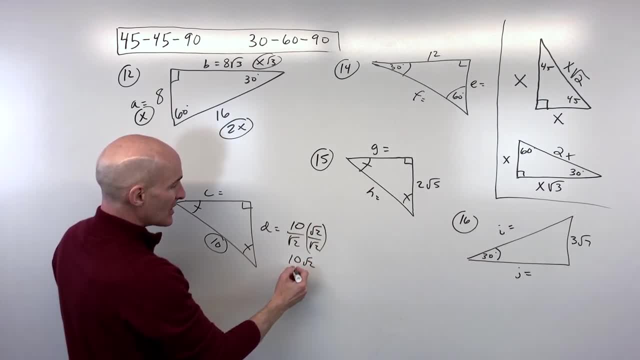 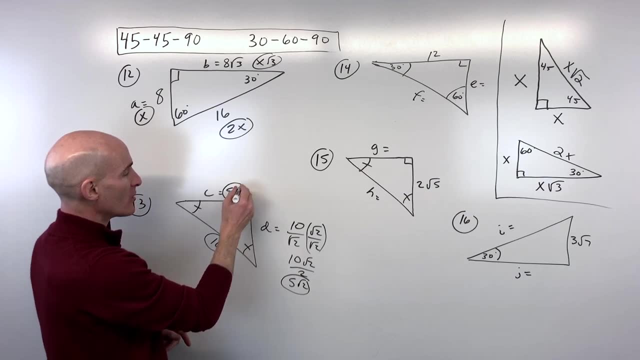 want that squared in the denominator. so we're going to rationalize: so 10 root 2 over 2, and the 10 and the 2 reduce so that comes out to 5 root 2. so both of these legs, remember they're congruent. 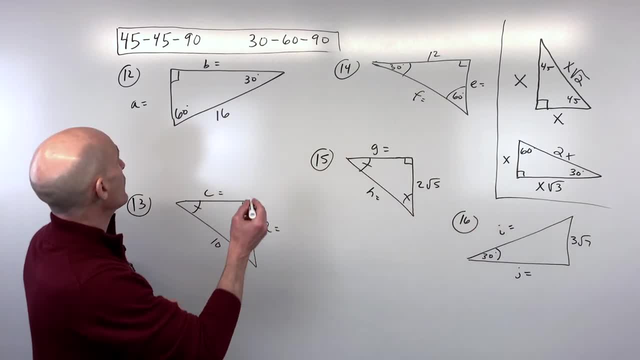 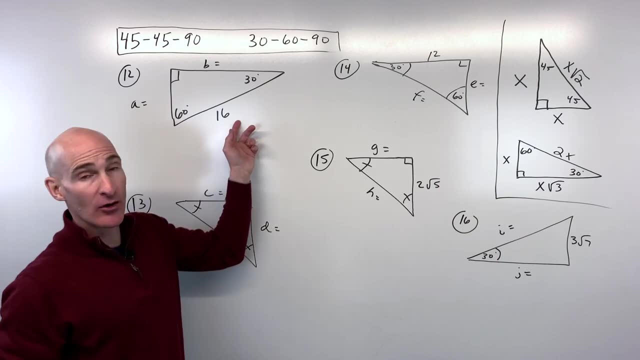 comfortable if you're used to seeing it in a particular direction. But what I like to think about is, you know, short legs across from the 30,, long legs across from the 60, hypotenuse is across from the right angle And, if you want to use that little technique I was talking about, 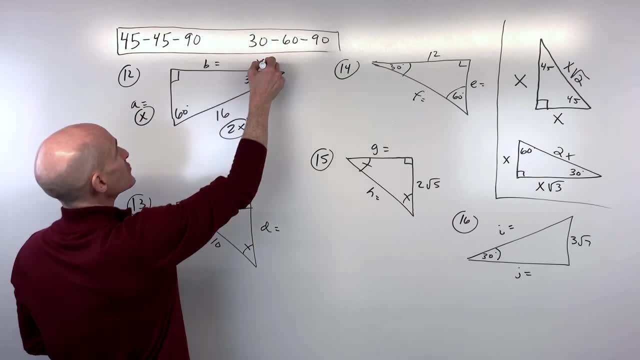 earlier with the 2x, 1x and x root 3 to kind of guide you. you can go ahead and do that. You can say: well, hmm, they're giving us the 2x side. I want to go back to the 1x side, so I have to divide. 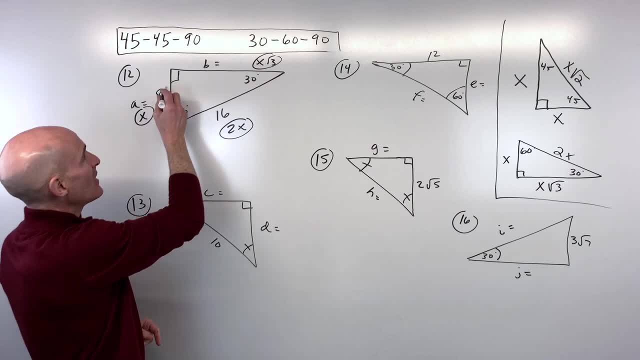 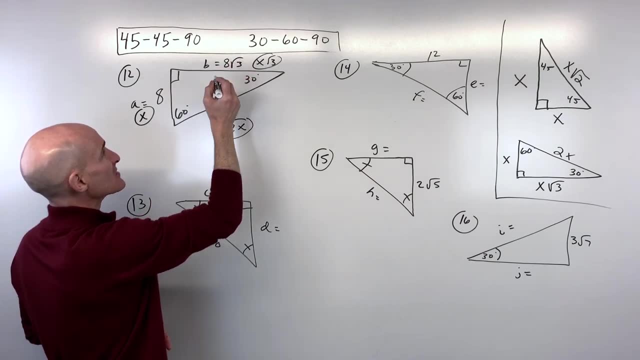 by 2.. What's 16 divided by 2? That's going to be 8.. Now to go from x to x root 3, I just have to multiply by square root of 3.. So 8 times square root of 3 gives us 8 square root of 3.. For number 13,: 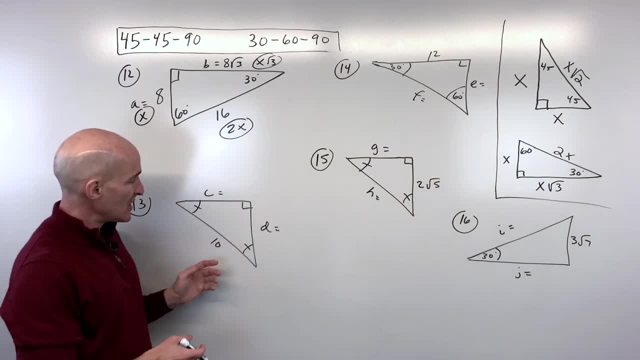 this you can see is a 45-45-90 triangle. Also, I rotated it a little bit to make it a little bit more challenging And you can see they're giving us the hypotenuse That's going to be our x root. 2. side To get that. you're going to have to rotate it a little bit to make it a little bit more challenging And you can see they're giving us the hypotenuse. That's going to be our x root 2 side to get. 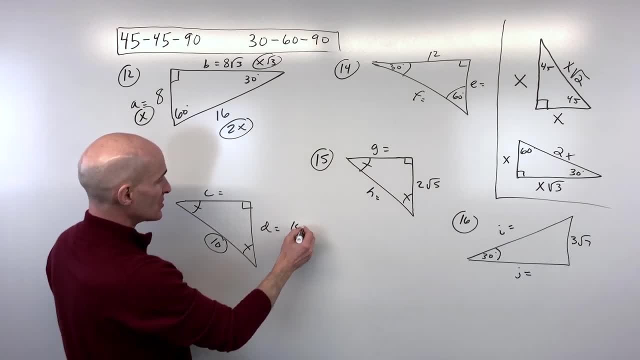 back to the leg. we have to divide by the square root of 2.. So it's going to be 10 divided by square root of 2.. Remember, we don't want that square root in the denominator, so we're going to rationalize. 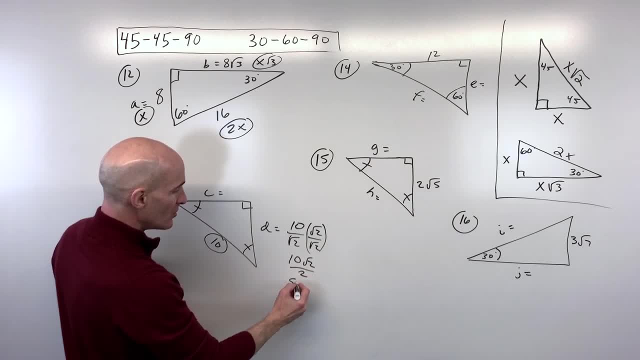 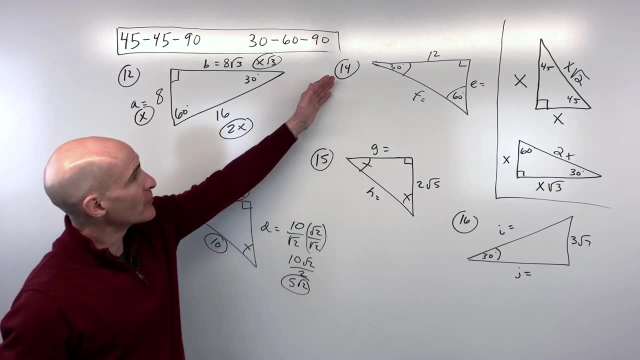 So 10 root 2 over 2.. And the 10 and the 2 reduce so that comes out to 5 root 2.. So both of these legs- remember they're congruent- are going to be 5 root 2.. For number 14, another 30-60-90,. 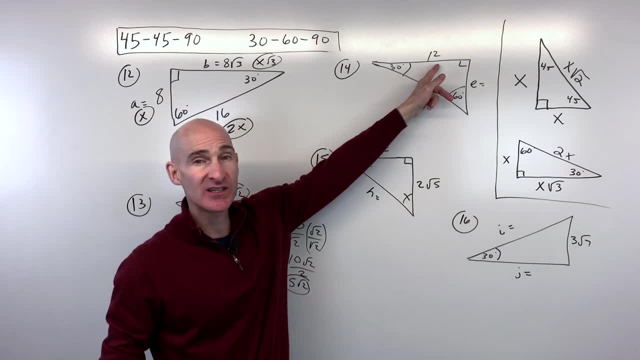 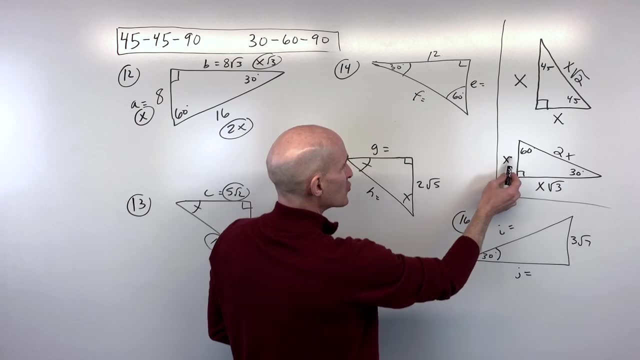 but what are they giving us here? It looks like they're giving us the one across from the 60 degree angle. That's our longer leg, That's our x root 3 side. Always with the 30-60-90, I always want to make my way back to the short leg. So I say, well, how do I get from x root 3 to x? 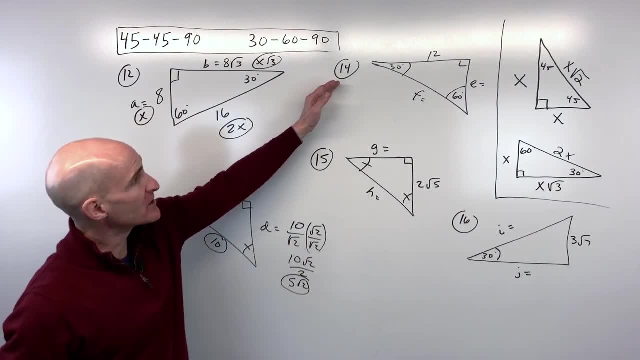 are going to be 5 root 2.. For number 14, another 30-60-90. but what does that mean? It's going to be 5 root 2 over 2.. So what are they giving us here? It looks like they're giving us the one across. 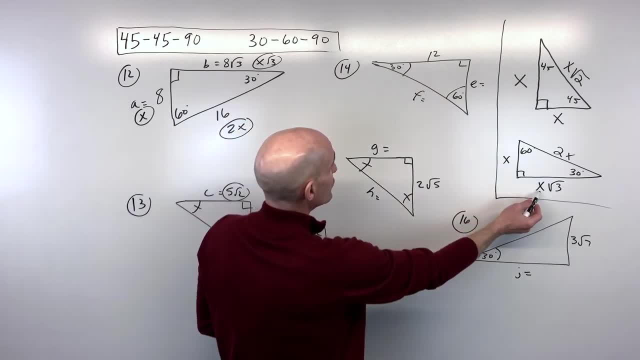 from the 60 degree angle. that's our longer leg, that's our x root 3 side. Always with the 30-60-90, I always want to make my way back to the short leg. so I say, well, how do I get from x root 3 to x I? 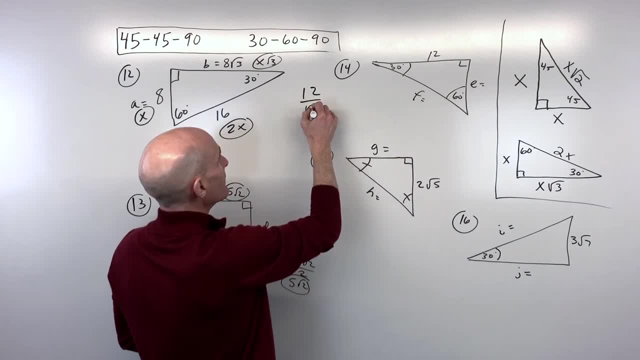 have to divide by square root of 3.. So let's see 12 divided by square root of 3. we don't want that square root of 3 in the denominator, so we're going to rationalize that gives us 12 root, 3 over 3.. 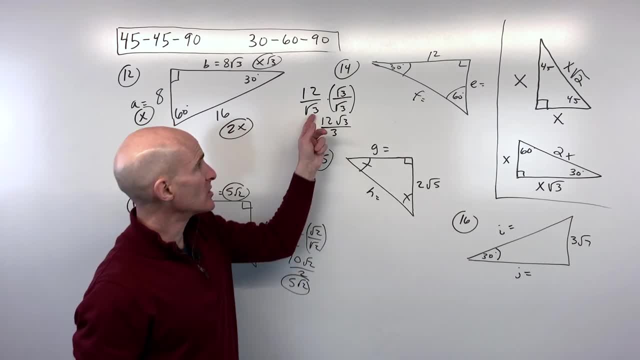 Notice, when you multiply a square root times itself, you get that number underneath or you can do: square root of 9 is 3.. The 12 and the 3 reduce the square root of 3 and the square root of 9 is 3.. 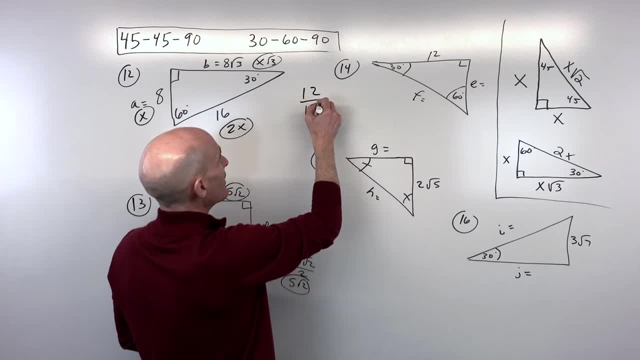 I have to divide by square root of 3.. So let's see 12 divided by square root of 3.. We don't want that square root of 3 in the denominator, so we're going to rationalize That gives us 12 root, 3 over 3.. 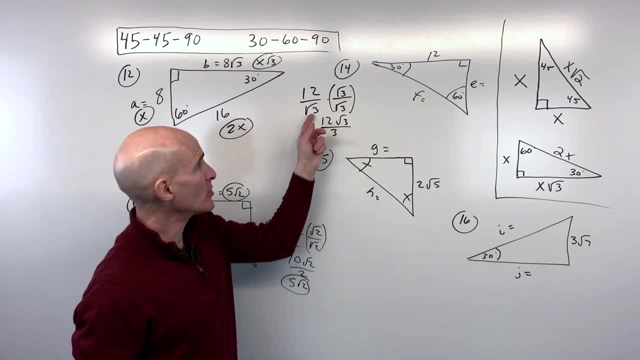 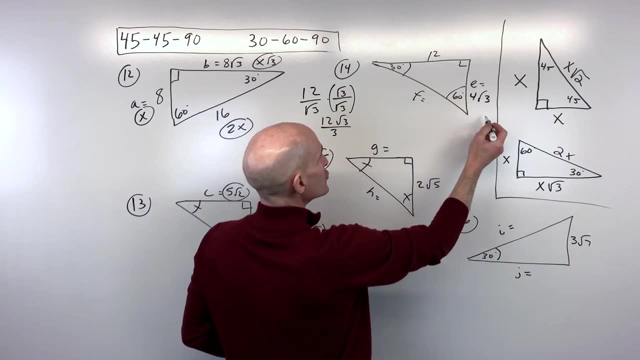 Notice, when you multiply a square root times itself, you get that number underneath. Or you can do square root of 9 as 3.. The 12 and the 3 reduce. so you can see we're going to get a 4 root 3 for the short leg. Now to go from the short leg to the hypotenuse we just have to double. 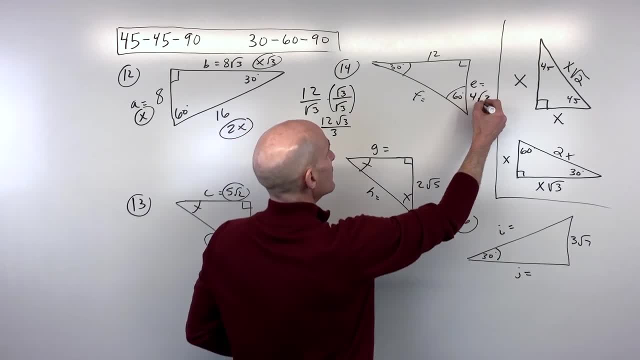 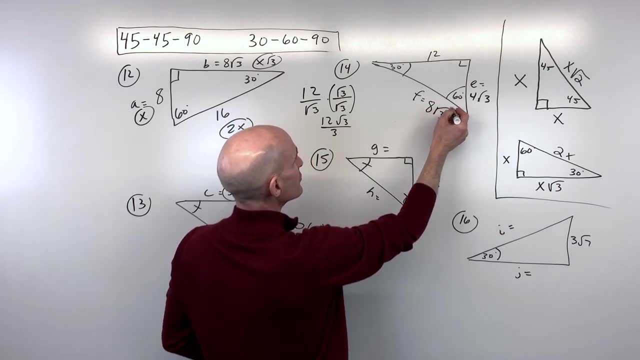 So you can see we're going to get 4 root 3 for the short leg. Now to go from the short leg to the hypotenuse we just have to double: 4 root 3 times 2 gives us 8 square roots of 3.. Okay for number 15. 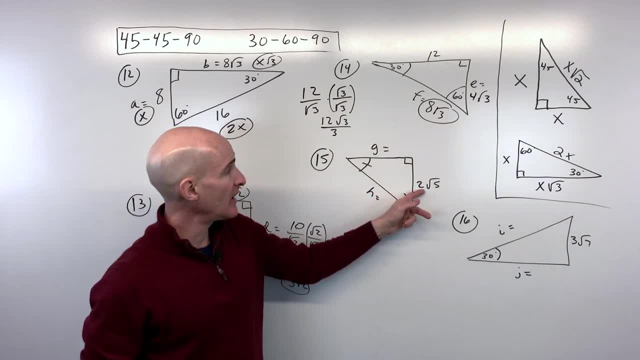 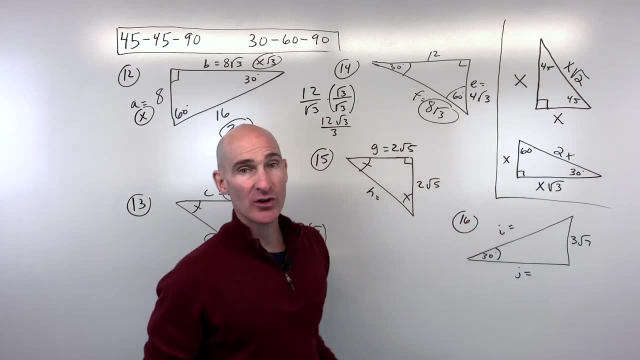 this is another 45-45-90.. It looks like we're given the leg, which means we automatically know the other leg is the same 2 root 5.. To get to the hypotenuse, though, we have to multiply by the square root of 2.. Remember, it's about 1.4 times longer, So if we multiply 2 root 5 times square, root of 2, we get 4 root 3 over 3.. So we're going to get 4 root 3 for the short leg. Now to go from the short leg to the hypotenuse, we just have to double. 4 root 3 times 2 gives us 8 square roots of 3.. Okay for. 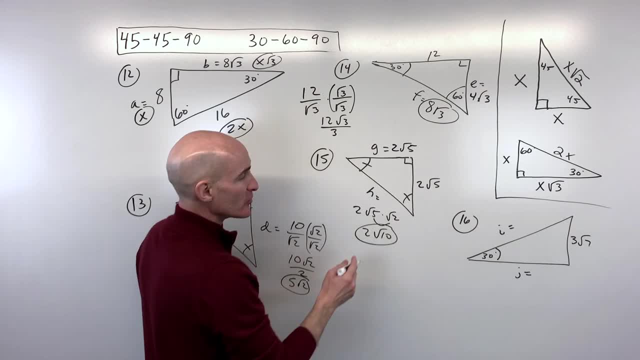 number 15. this is another 45-45-90.. That's going to give us 2 square root of 10.. We want to multiply those square roots together. And then, the last problem, another 30-60-90.. Let me see if I can. 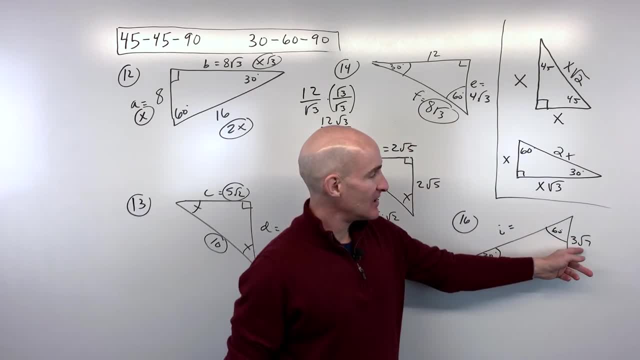 finish drawing that 30-60-90.. Looks like we're being given the short leg, the one across from the 30 degree angle. So to get to the hypotenuse we have to double it. So that's going to be 6. 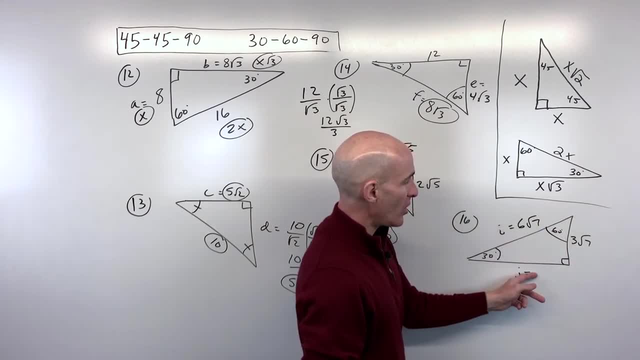 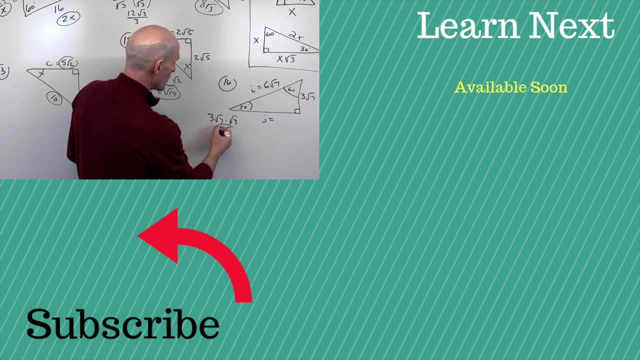 square root of 7.. Okay, and then to go from the short leg to the longer leg, we have to multiply by the square root of 3.. So 3 square root of 7 times square root of 3 gives us 3 square root of 21.. 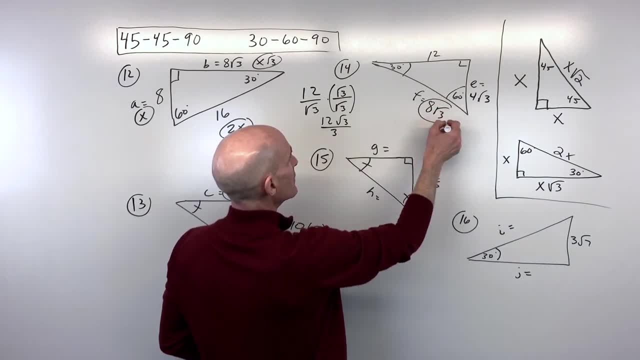 it: 4 root 3 times 2 gives us 8 square roots of 3.. Okay for number 15, this is another 45-45-90.. It looks like we're given the leg, which means we automatically know the other leg is the same. 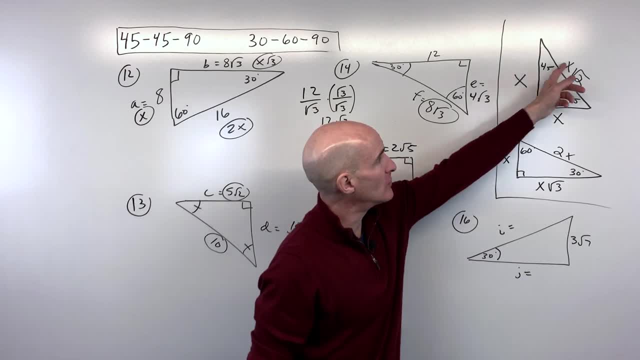 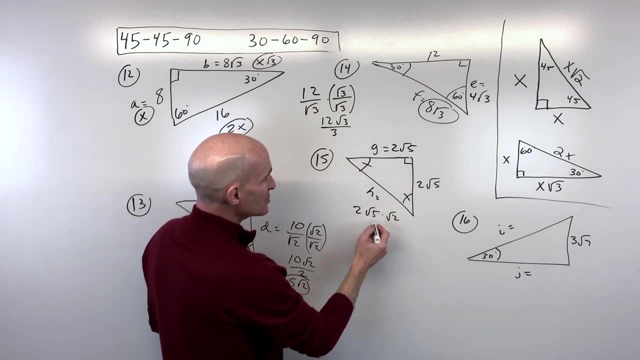 2 root 5.. To get to the hypotenuse, though, we have to multiply by the square root of 2.. Remember, it's about 1.4 times longer. So if we multiply 2 root 5 times square root of 2, that's going to give us. 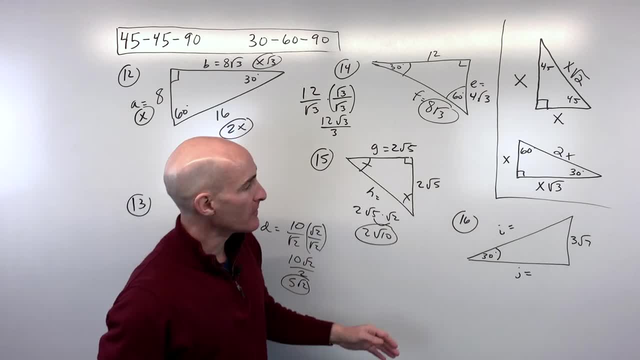 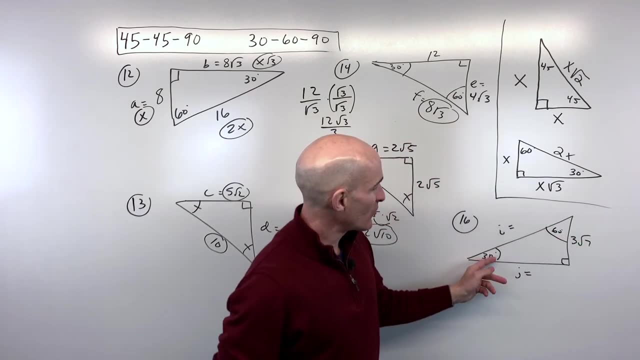 2 square root of 10.. We want to multiply those square roots together. And then, the last problem, another 30-60-90.. Let me see if I can finish drawing that 30-60-90.. Looks like we're being given the. 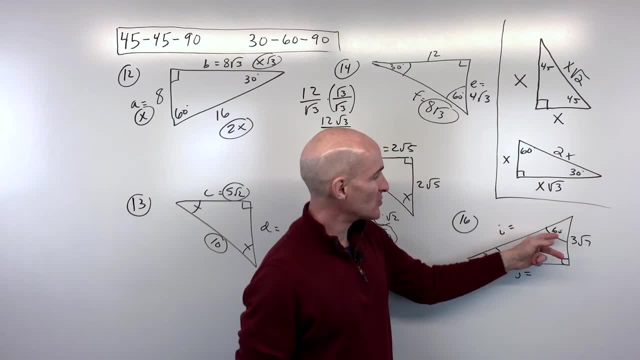 short leg, the one across from the 30 degree angle. So to get to the hypotenuse we have to double it. So that's going to be 6 square root of 7.. Okay, and then to go from the short leg to the 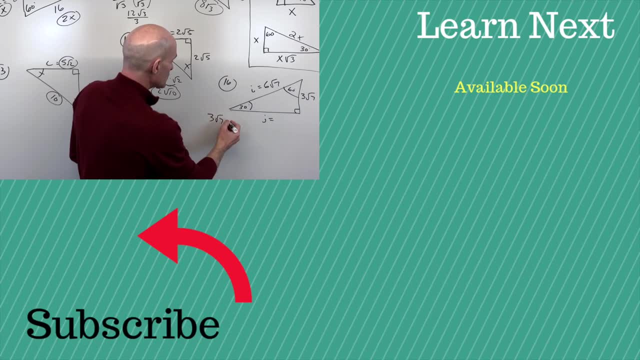 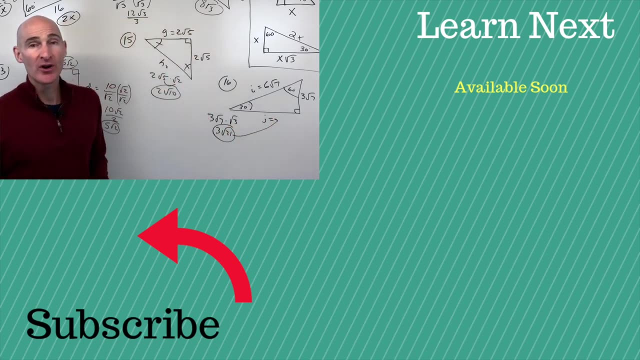 longer leg. we have to multiply by the square root of 3.. So 3 square root of 7 times square root of 3 gives us 3 square root of 21.. And you got it. So I hope you enjoyed this video, If you. 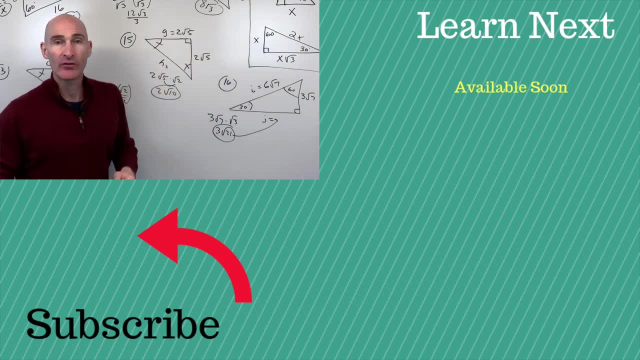 want to see more examples. I'll put a video up there that you can check out for more practice, more examples with 45-45-90-30-60-90.. I look forward to helping you in the future videos. I'll talk to you soon.